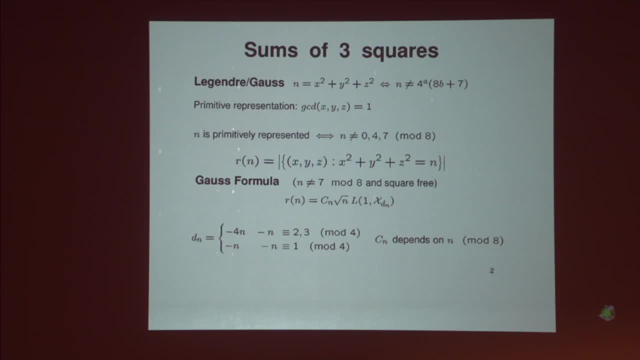 on n mod 8, times square root of n times the value of a Dirichlet L function at the point 1, the Dirichlet L function which is associated to the Dirichlet character given by the square 3, and the Kronecker symbol associated to the n, which is defined below. 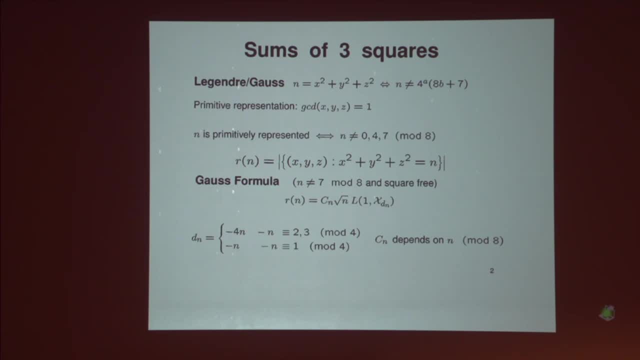 Well, at some point we will use this exact formula, but for the time being, let me just say that this special value of this Dirichlet L function at 1 can be evaluated from below using zero and for both, And what it tells you is that next slide. 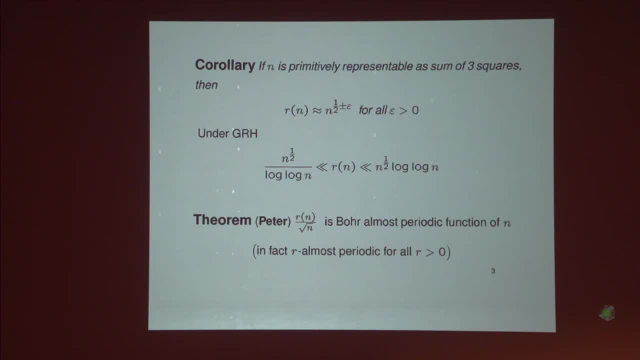 So this is the Dirichlet L function at 1.. This is the Dirichlet L function at 1.. Next slide: Rn is roughly, like I said, square root of n up to a factor which is of the order of. 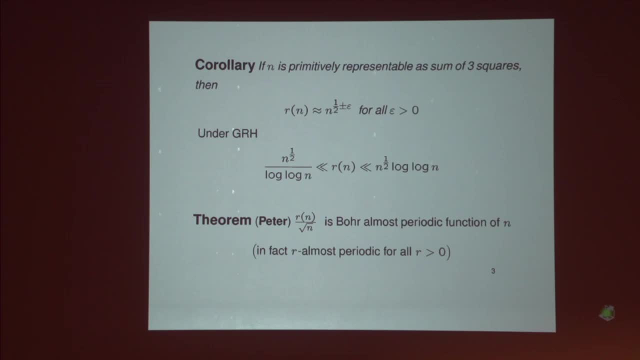 n plus or minus epsilon. So Rn is bounded from above by n at the power of half plus epsilon, and from below n at the power of half minus epsilon. plus or minus epsilon. and that assuming that n is primitively representable as a sum of three squares, 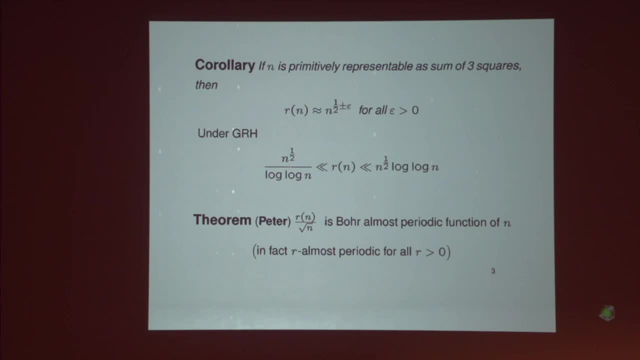 Now, under GRH, The n is a constant. The epsilon can be replaced by the block n. So what we see is that, like I said, Rn is roughly like square root of n, but there is a certain fluctuation. 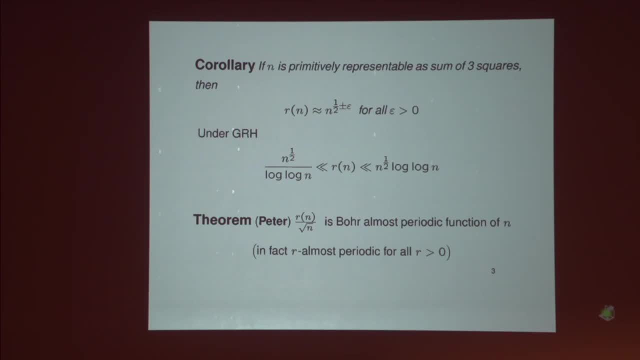 Now one can get more into details about these fluctuations and factor the theorem by Peter- not Peter Sarmack, somebody whose last name is Peter. Please look at this Now: if you normalize Rn by square root of n, you have an almost periodic function in. 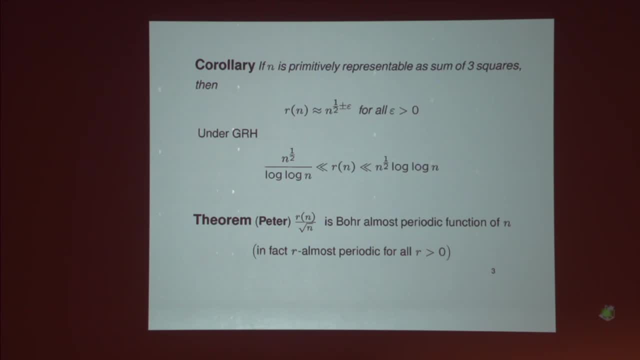 the sense of Bohr, And in fact it's also a far almost periodic function for R In particular. R is a bad notation here. I should say k. If you take any power of Rn over square root of n, the average is over n unbounded. 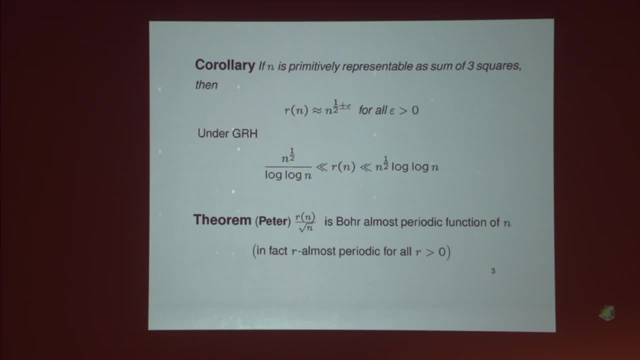 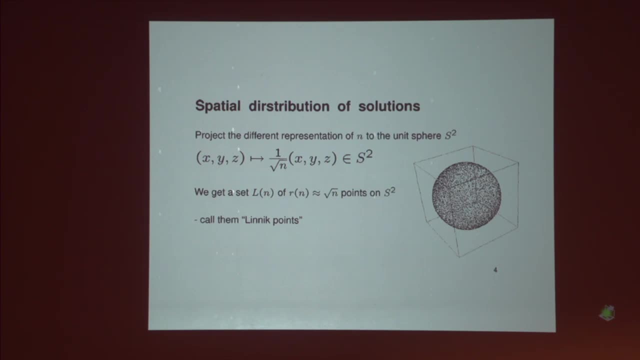 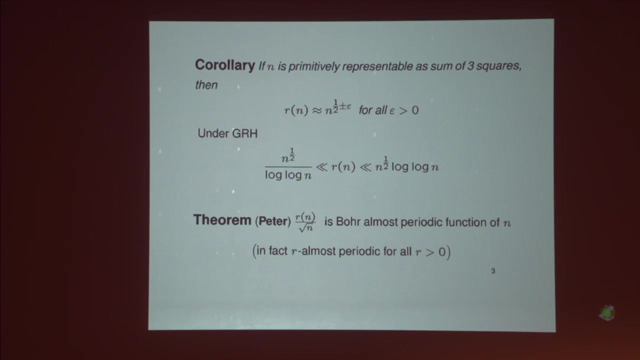 This is also something that we play about later on. What I should point out is that the treatment of representations of an integer as a sum of these squares is not something which can be handled by the circle method, unlike in the case of sense of Bohr squares, where one can apply the Klosterman version of the circle. 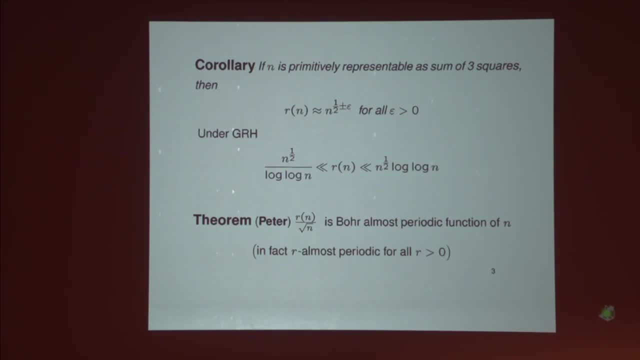 method. Or five squares, the sums of five squares, et cetera. So it's not something that can be handled by the circle method. So it's not something that can be handled by the circle method. So it's not something that can be handled by the circle method. 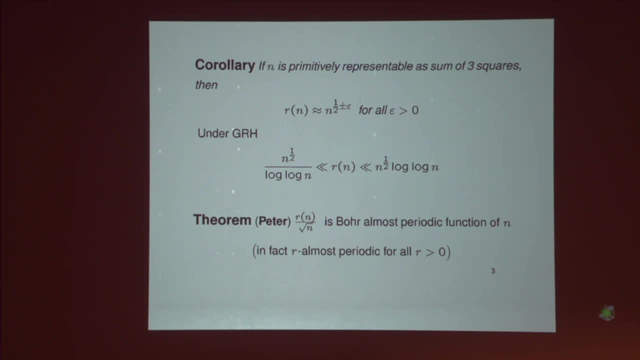 We have used the K-tomb function, but we also have a little bit of the K-tomb function and the three squares, et cetera, which is how the little root, And so for sense of three squares, this is something which is more intricate. 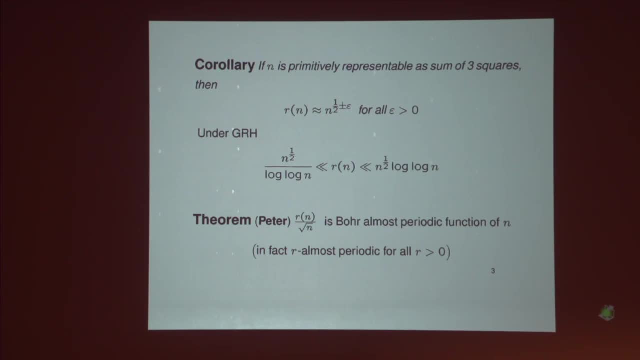 Nevertheless, the theorem of almost periodicity, which I've heard as a speaker's theorem, this is something that can be proven. This is not too difficult using certain method considerations. So what we have there is a large set of representations. 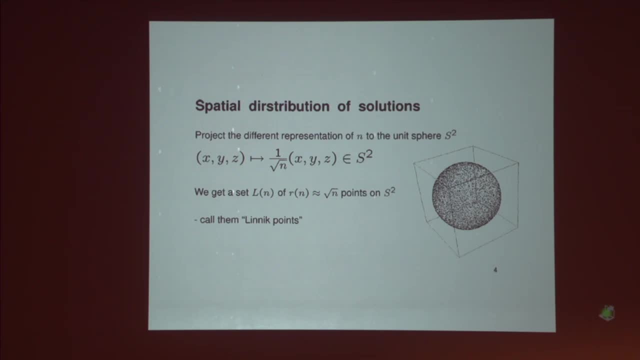 So next slide. The question was: is there a characteristic feature in the decision-making mechanism that we are? the general question we're emphasizing is what is really the distribution of these different representations? so what makes sense is to put everything on the unit sphere. so remember. 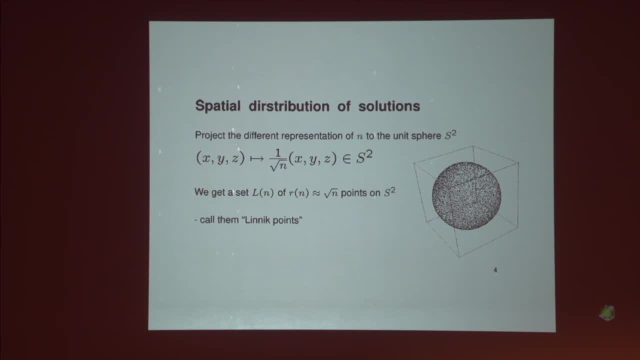 since x squared plus y square plus e squared is equal to n. what we have there are vectors of the cleanly known square root of n, so the square root of n, and we get the point. we get points, in fact we get rn points on the units here, and then we can ask for the distribution of these. 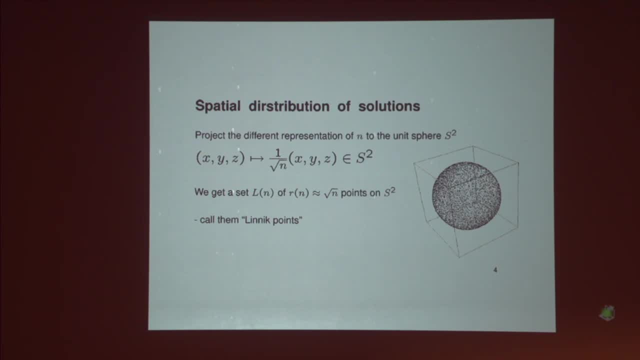 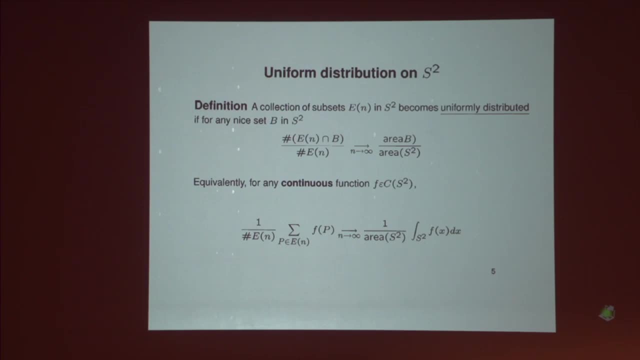 plots. we will call the set of these points, we will call them meaning points, so we can study. next, next one: we can study the distribution of this limit points at several scales. so the cross scale is what corresponds to uniform distribution. so let me remind you that the collection of subsets 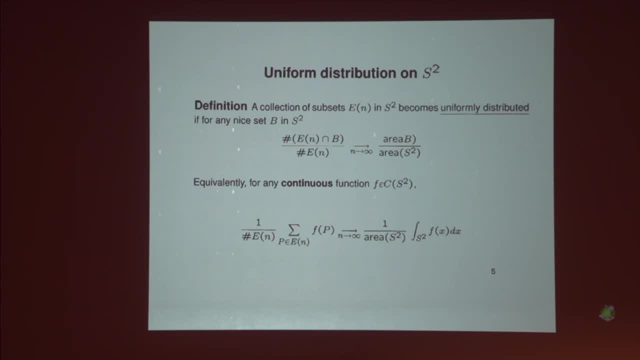 e, n in the unit sphere is uniformly distributed, provided if we take a, nice and b is two. so we are basically not going for very small sets. we're taking sets, say, which are the order of say, say order one, and which are nice. we're looking at the ratio between the number of 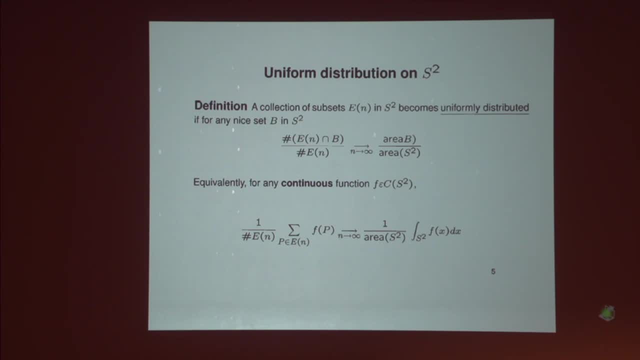 points in the set e n. so the number of points from the set e n to b, the ratio versus the total number of points. what we'd like is that, from n going to infinity, this converges where to where it should be, which is the relative area of that set b, or equivalently we can define it. 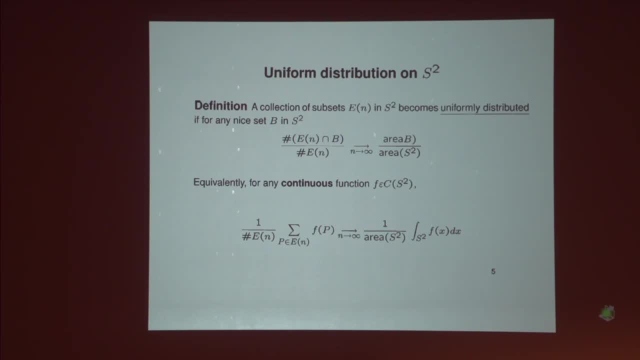 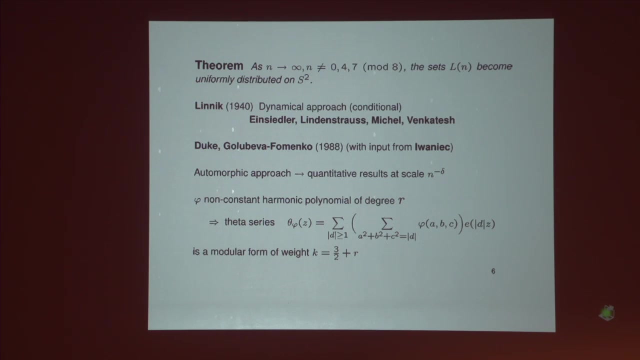 by averaging continuous functions on the sphere, by averaging continuous functions of the discrete sets e, n and requiring that this converges to the, the big average of the function f. now what happens with limit points? next slide, next slide. so what linit foremoved, partly conditionally, is that? so we're making the assumption that 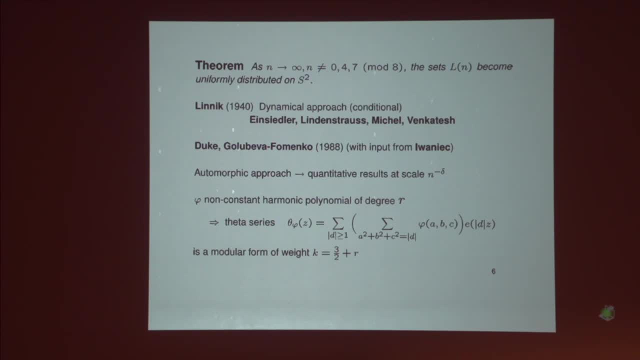 n is not zero: four, seven more eight- and goes to infinity. so we're looking at these link points and there is a deep theorem which is due to linic. 1940 tells you that indeed, this, this sets of points, became eq distributed. so, like i said, this was slightly conditional. 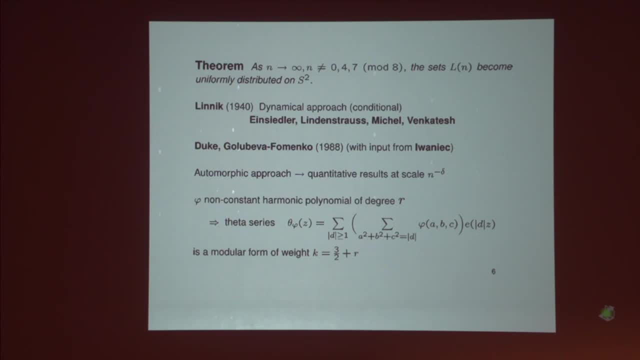 what linic uses is. the narcotic approach is a dynamical approach which was later presented in an unconditional and modern form, in fact relatively recently, in the work of and cedar and cedar in the store special in venkatesh. what they should point out is that ergodic techniques are extremely powerful in order to 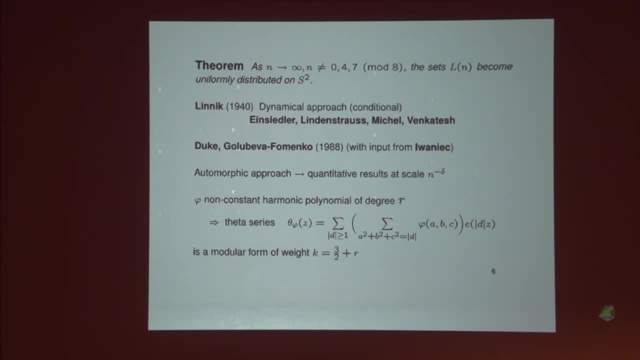 detect, to establish qualitative phenomena, but usually they do not offer any kind of quantitative insight. so when it comes to quantitative statements, usually they do not. they do not perform well. on the other hand, for our discussion we will need results which are slightly more quantitative, and there is an important breakthrough there. 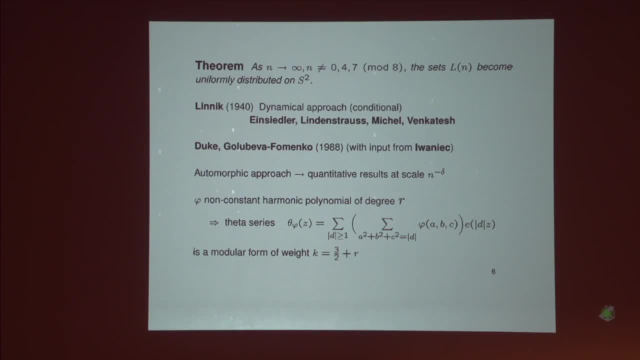 which goes back to energy advantage and then applied in that particular setting, independently by the duke, and which is a completely different approach to this distribution, which is the automatic approach. and this automatic approach has the advantage of giving you quantitative results about the distribution that works up to scale n minus delta. for some, 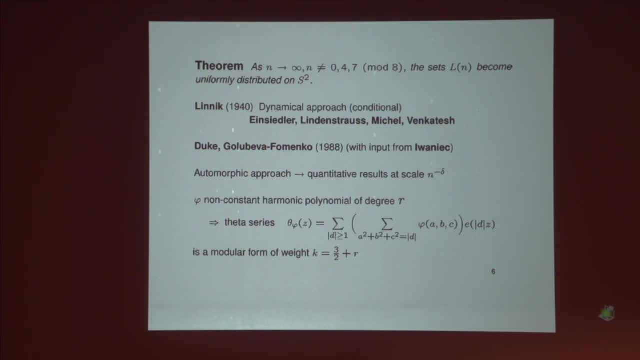 small, uh, delta, i don't think anybody knows exactly what is the best one. one can do that. i'm relatively small. the main thing for us is that you can reach some kind of power gain there. so the basic idea of the automatic approach is that when you test a eki distribution using harmonic polynomials, 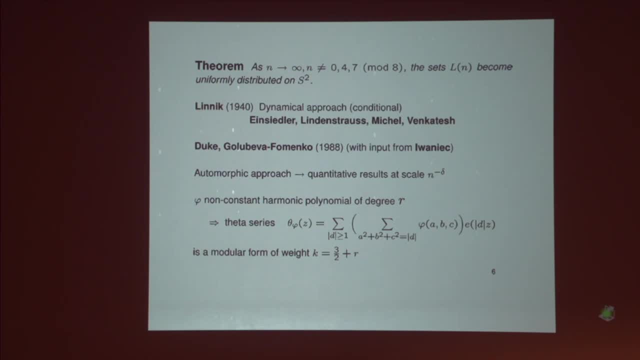 on the sphere. so there is an important point. there is that if you start from a non-constant, constant harmonic polynomial of degree r, you can construct a theta function from there and basically the full coefficients of the theta functions, of the theta function, they give you exactly the quantity, the quantities you want, namely the average of that harmonic polynomial. 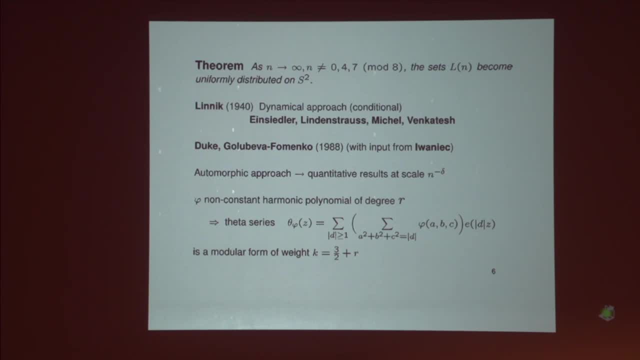 over. this is like this point. so the d fully coefficient is just the sum of the harmonic polynomial five a, b, c over all. a b, c satisfying a squared plus b squared plus c squared d. so that is exactly what we want to control. getting it into distribution amounts to getting it not to bounce. 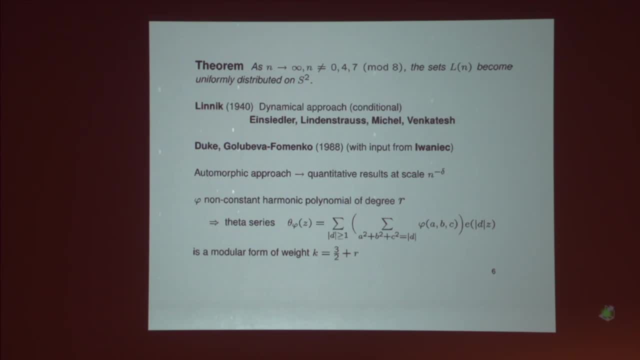 on these coefficients. and well, what it turns out is that this data series is a model of form, and then one can use the theory of model forms to get down to bounce on these coefficients and eventually this leads to quantitative, to quantitative results about distribution, because, basically, if you have a certain certain set gap, you can approximate. 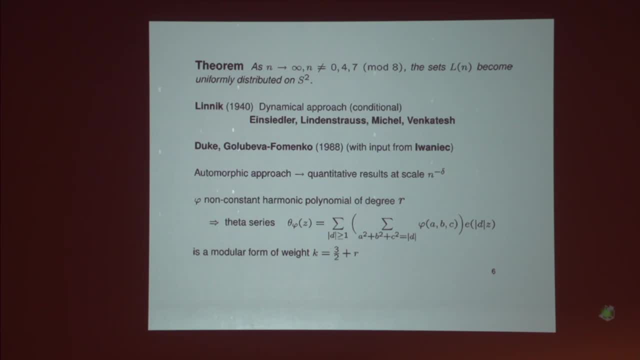 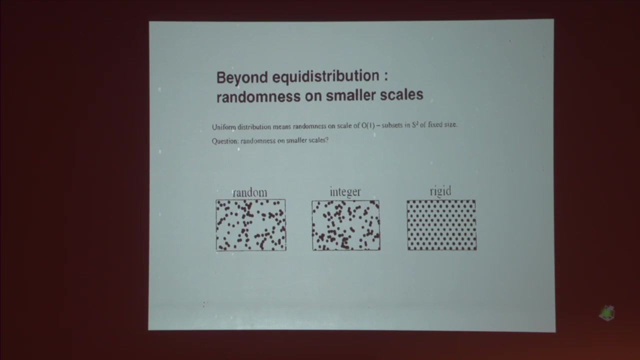 in some sense the indicator function of this gap using harmonic polynomials, and then you can use the filtrate of this data to distribute theTS Lesion on this average, the harmonic. now this on this. on this last point, next slide right. so in any case, again, this story is about distribution. its anything Sh네hengecог facts. what you're telling about distribution is something that can be handled with two quite different techniques. one technique is the toch diagnostic and tactical way that was used a lot in the pilot translation techniques. so one technique is the vertical technique and the other technique is the conduct. 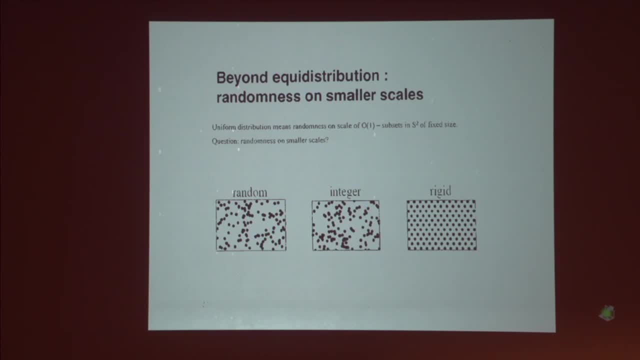 is the ergodic technique. the other technique is the autonomic technique, but again, there is no, there is no. weight is no, no approach norm, simply via a certain method, as is possible for more variables. so this is what happens at the very core scale. now i would like to go to finer scales. 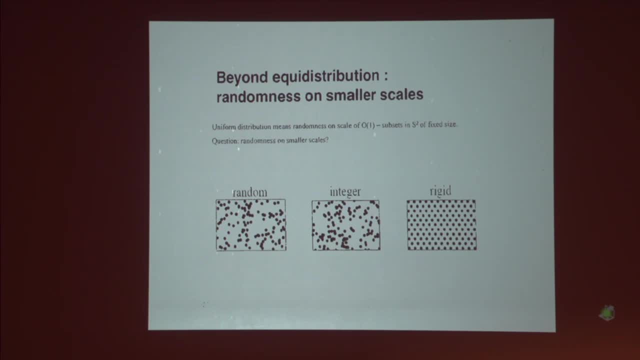 you will have sets which are uniformly distributed on the final scale. they still can have quite different behavior, because you can realize- you can realize icky distribution in a rigid way and you can also realize distribution in a random way where basically the, the forms are produced by some process. now there have been 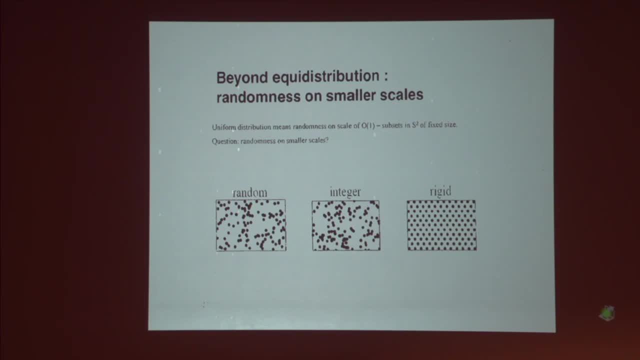 this kind of studies. there have been quite serious numerical checks on what happens with leading points, and these leading points on small scale. they seem to also on larger scale, but they seem to indicate a behavior which is like the random behavior opposite to the rigid behavior. and what this talk is basically about, and this is basically about is 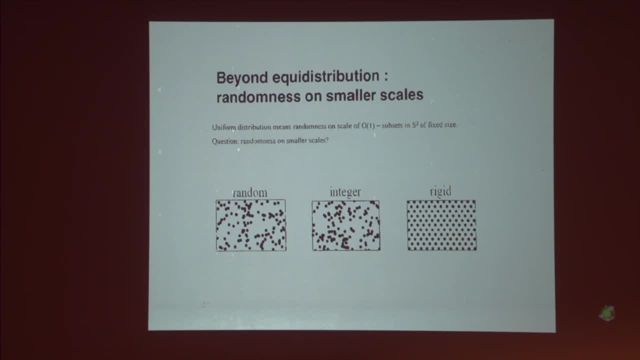 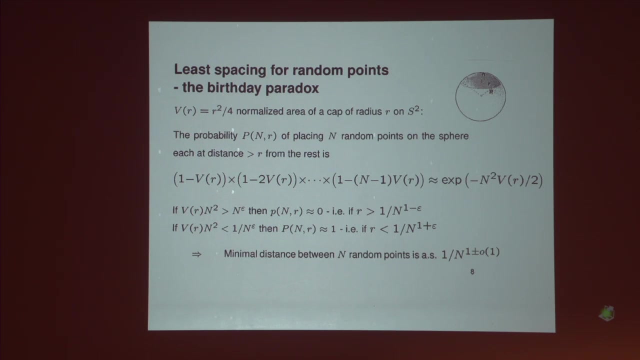 to find, uh, rigorous uh, is to prove rigorous results that somehow support this random behavior. next transference, next slide, next slide. okay, so the what one you should ask probably, is why we really focus on terms of three squares. well, all the evidence from what they said before is that treating center, of course, pairs or more. 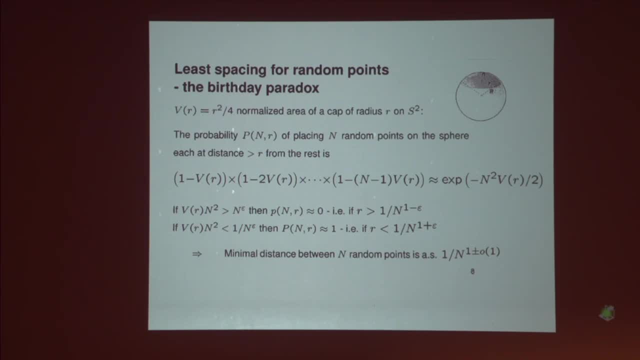 and understanding the distribution of these representations is much easier. so, first of all, let's say that you were fixated with this idea of random behavior, and there is a reason why this, this model of link points, somehow is the only one that can be compatible with the random behavior and the effect. uh, what is going on is that 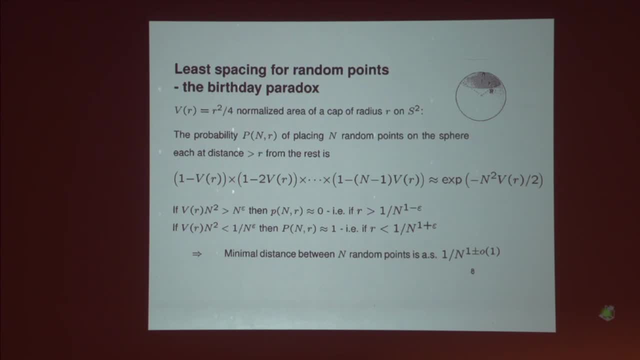 when we have more barrels, when we're taking sets of hot squares. there is a problem if we want to implement the random model, and this problem is actually quite simple. it has to do with the per se paradox, namely the lease spacing for random points. what it turns out is that 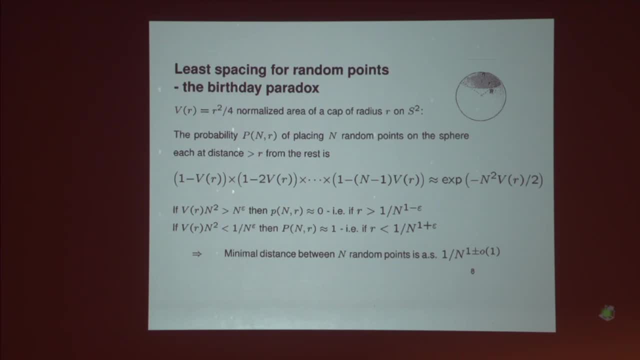 uh, when we're taking, when we're一定要, when we're going to higher dimensions, the separation between the points, the obvious separation, is not compatible with the random model which predicts minimal spacings, which are small. So let me be a little bit more clear about that. 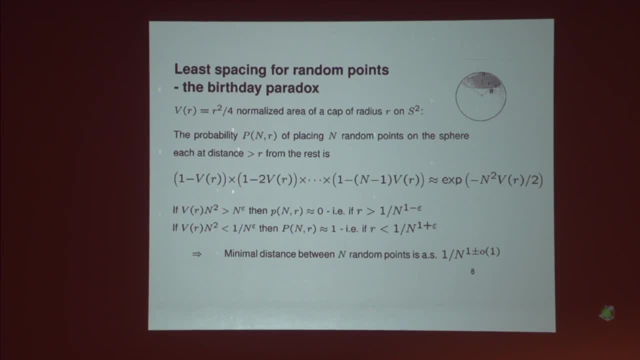 So what we're doing is that we are considering the area of a normalized area, of a cap of radius r on the two spheres, which is like r squared, And so this is the random model. Then we're taking n random points on the sphere capital, N random points on the sphere 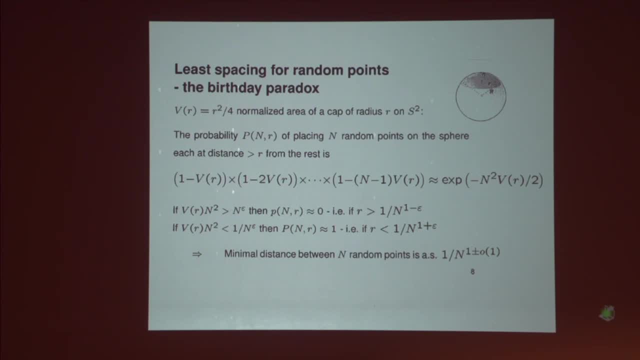 and we're asking for the probability Capital P and r. if we're placing this n random points on the sphere, then the multiple distances are all, say, strictly larger than r. So an easy calculation shows that the critical value of r is like one over capital N on the sphere. 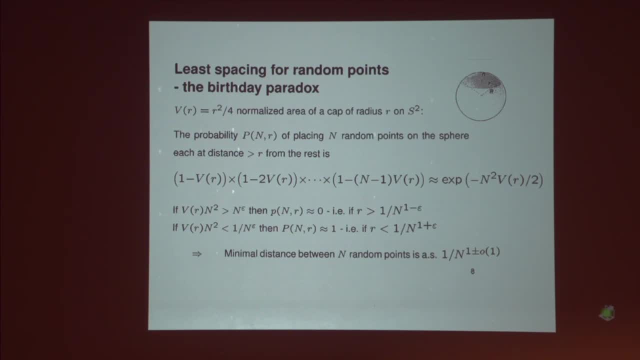 So, in other words, in this random model, what we're going to have almost surely are encounters which are, say, pairs of points which are at distance of the order of one over N, one over capital N, If we translate that to the original set of representations. 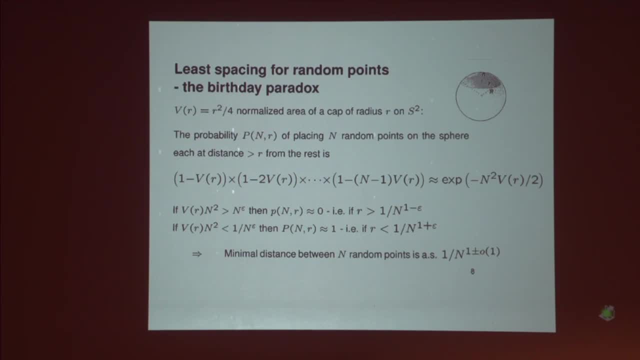 so the number that we scaled everything down to the unit sphere. now let's go back to what happens with representations: n equals x squared plus y squared plus c squared. So we have to multiply everything there with square root of n, And so what it turns out is that this capital N is roughly square root of equal n. 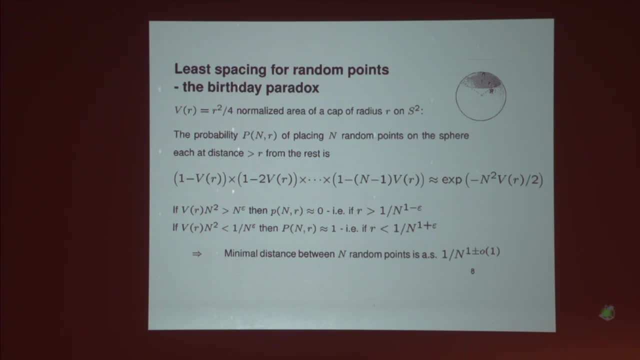 What it turns out is that the separation of one over capital N on the level of S2 corresponds to a separation which is O1 on the level of the representation. So it is completely clear that if you have distinct lattice points, the distance is always at least equal to one. 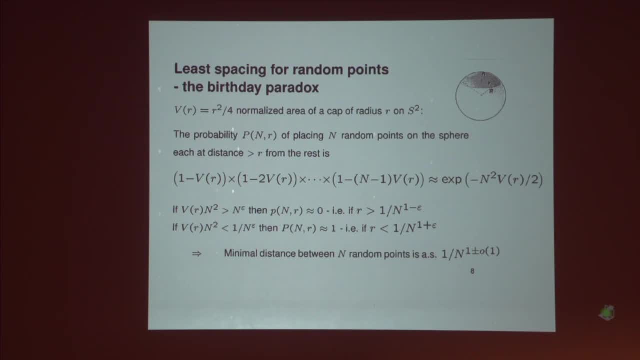 So, from that point of view, there is no incompatibility with the random model. On the other hand, if we go to higher dimensions, say dimension four, and we are again examining the Birzweil paradox, what you see? so, instead of r squared, get r cubed. 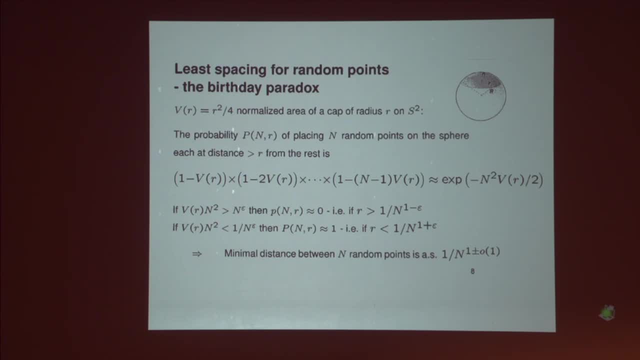 then the number of points. there the capital N is not going to be like square root of n, but it's going to be like n. So if you check what it means eventually, you see that the random model would predict that on the level of the lattice points, 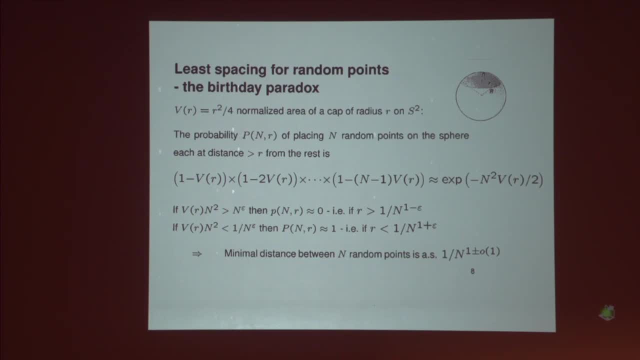 you would have different points which are a distance much closer than one, because what it is is n minus one over six, or something like that, And we know that this is simply not the case, because there is a figure with a lower bound, which is O1.. 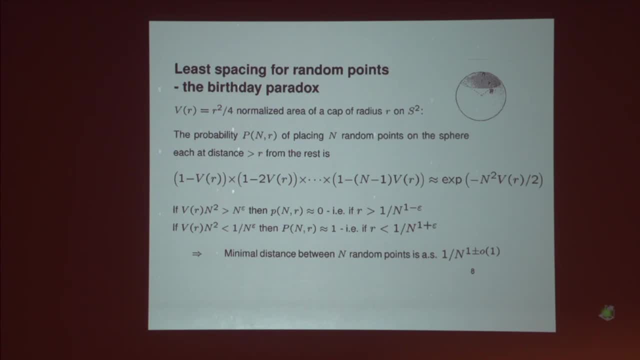 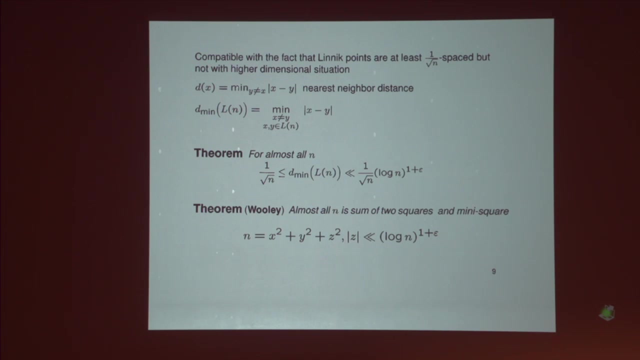 So, in the same sense, that point of view rules out higher dimensions as a possible candidate to claim any kind of random behavior. Next slide, please. Next slide, Yes, Okay. So let me summarize that What we are doing is, for each point x of each limit point. 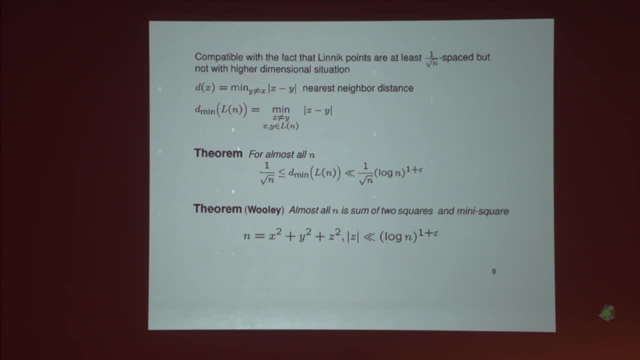 is to take the distance dx to the nearest point y different from x, and then we take the minimum of, so d min of that set. Ln is the minimum of dx, so in other words, the minimum of the distances between points x and y. 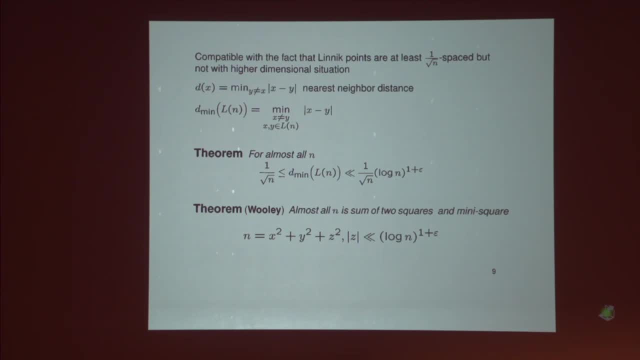 in the set with x distance from y. So previously what we saw is that d min of the Ln set points is going to be at least one over square root of n, which is compatible with the random model. The random model predicts also that this d min is in fact on the part of one over square root of n. 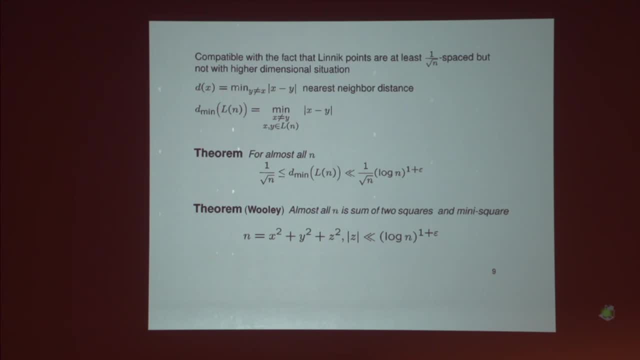 Now that we can show for almost all n is f to the factor of n, using an interesting result by Trevor Woolley which says that almost all n can be represented as a sum of two squares and a minisquare, where the minisquare is basically of logarithmic size. 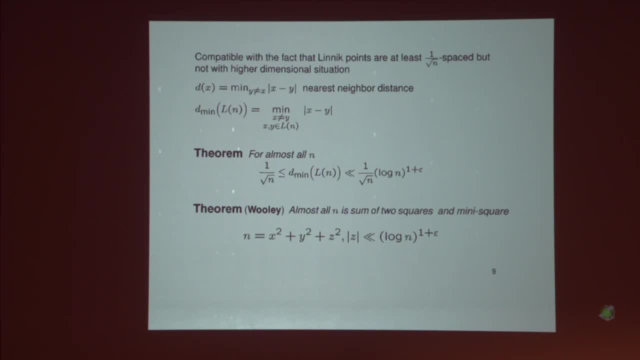 Now one could conjecture that there is a statement like that could be true not only for almost n, but for all n, with the minisquare being bound by n to the epsilon. But that turns out to be an extremely hard question. 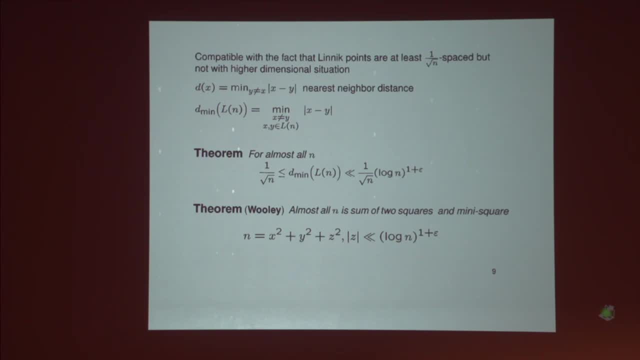 So, in any case, for almost all n, we have the behavior of d min, which is basically the random behavior. Next slide To get more specific. what captures the statistics of the distribution of configurations is a so-called Ripley function. 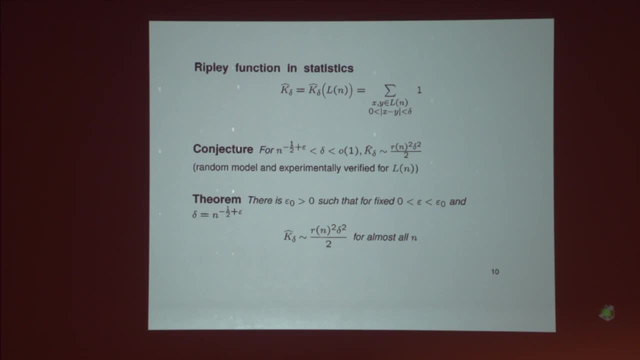 which is very simply defined as follows: We take k hat delta, which is the k hat delta of our set to be the number of points x- y in our configuration, x different from y and a distance at most equal to delta. 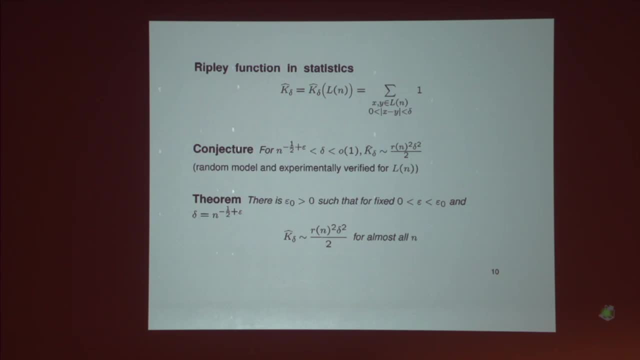 So the conjecture, which is what would correspond to a Poisson model, is that, basically, in the entire range of delta, the k hat delta behaves like r n squared delta squared over 2.. So this is what the random model predicts. 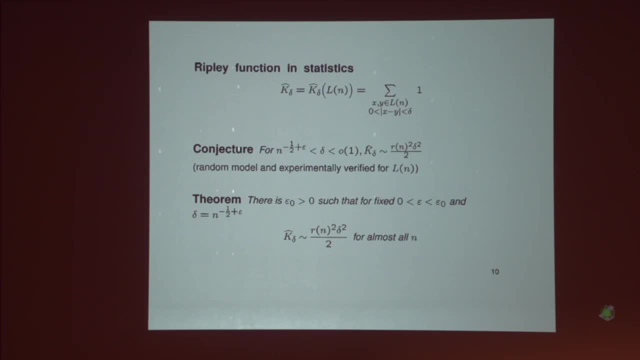 and that is what also experimentally, has been verified for r, n, for n. So what they will discuss are certain number of results that somehow support this projection. So the first result tells you that, on very small scale at least, for almost all n. 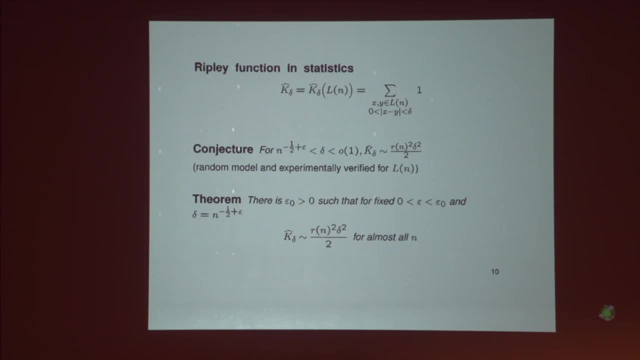 this behavior is correct. So we have that k delta hat is going to behave like r n squared, delta squared over 2, provided delta is sufficiently small. so we're assuming here. So this is really the size which corresponds to what I just discussed. 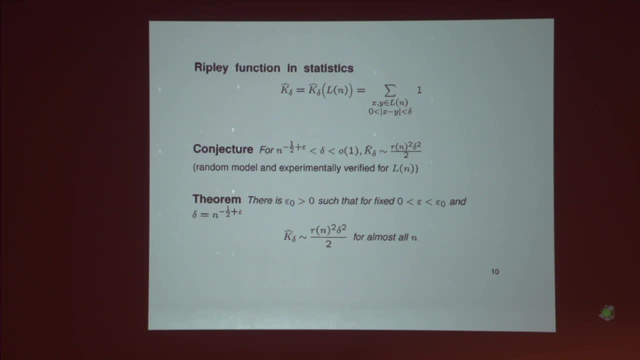 around the birthday paradox. n at the power of n is a half, as epsilon is less than epsilon zero. So in some sense this is already quite satisfactory from the point of view of justifying a Poisson-like behavior. is that this is what corresponds? 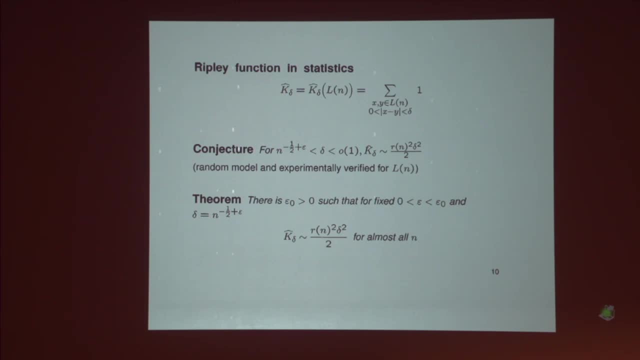 to the random behavior and definitely not the rigid situation, Then what we can show is that for all n the k hat delta satisfies the correct upper bound, at least slightly conditional. so there is a very weak conditional assumption there, which is the absence of z to 0,. 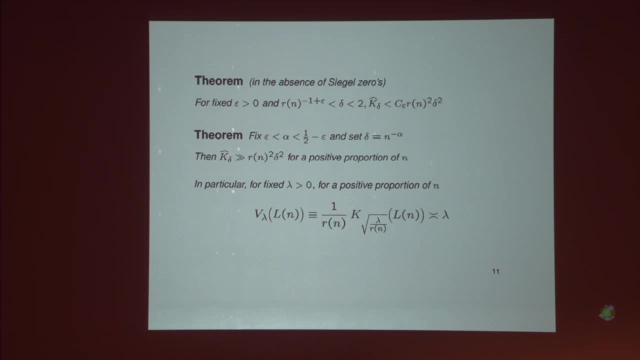 which is much, much weaker than the generalized thing, which is the same hypothesis in the sense that, well, if somehow, for some reason, you would have a z to 0 that would spoil the picture for some n, then basically it won't happen. 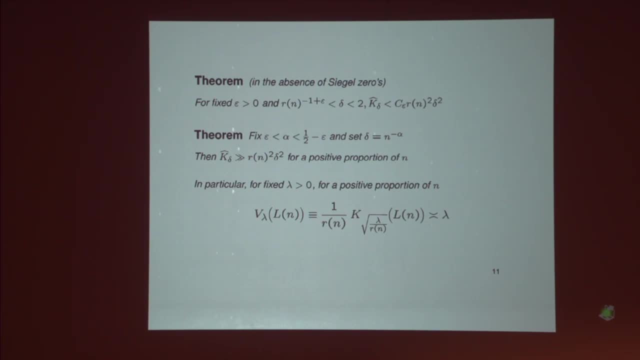 for all n except to be the isolated event. So that is for the upper bound. What is more interesting is the lower bound. So as far as the lower bound concerns, what we can prove is that we have the lower bound. 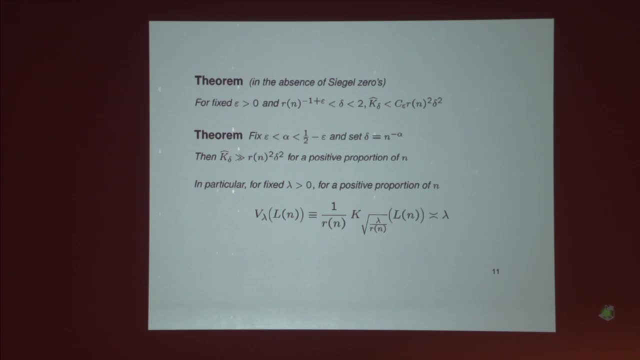 at least for a positive proportion of n. In particular, remember that the proof should say that the typical separation between limit points is the square root of 1 over rm. So what we can do is look in the window there so we can fix a lambda. 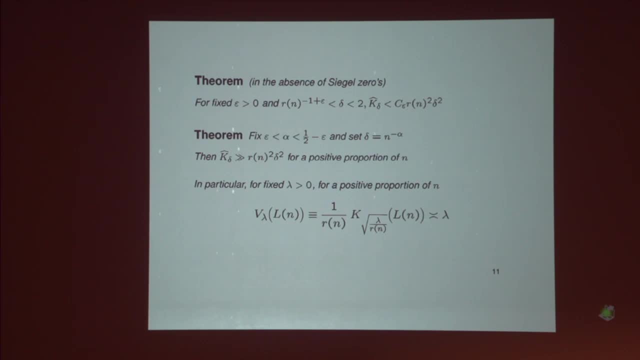 any lambda that's fixed, and then taking delta to be the square root of lambda over rm. What we see there is that the square root of delta, as predicted by the random model, should behave like lambda. Indeed, that is the case, and that is the case at least. 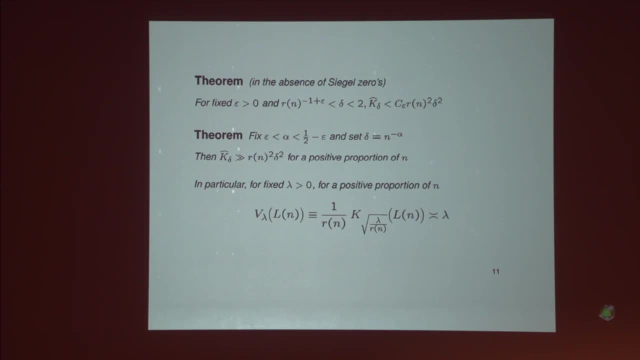 for a positive proportion. And this again is taking lambda small, fixed but small, clearly making the point of having a random behavior rather than a rigid behavior. because if the distribution would be rigid and we're taking lambda small, then the point it will describe. 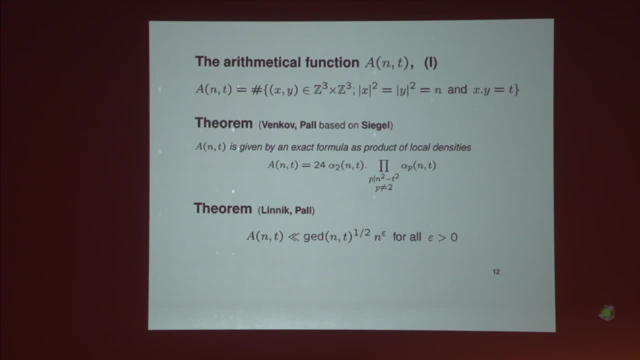 will be equal to zero. Next slide: Yeah, so I will not discuss the first theorem, but I will say some things about the second and the third theorem. So what is at the heart of the discussion? for the second theorem is an arithmetical function. 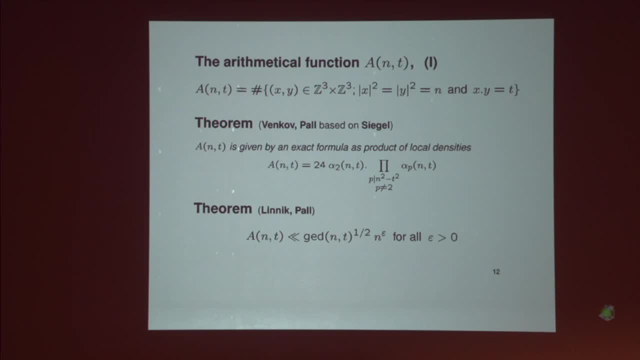 which I call a and t, and which is just so. a and t is the number of pairs, x, y, so integer vectors of, of norm, of square of norm that equals n and such that the dot product of x and y is equal to t. 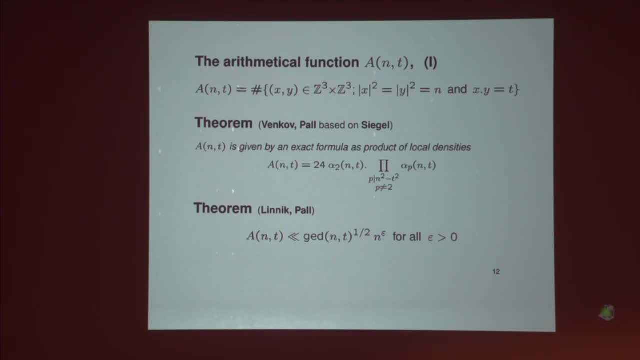 What is this dot product Interesting? well, if you write down the square of the distance between x and y, this of course can be expressed as 2n minus 2t. So, basically, this t is immediately relates immediately. 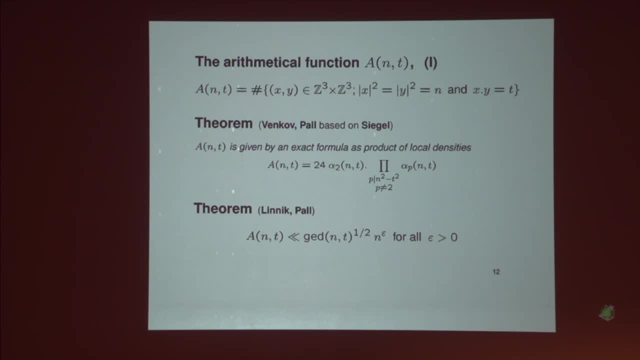 to the distance between x and y. So what we want to understand is this arithmetical function, and we will do that in several stages. So it turns out that there is a powerful tool to study this arithmetical function. 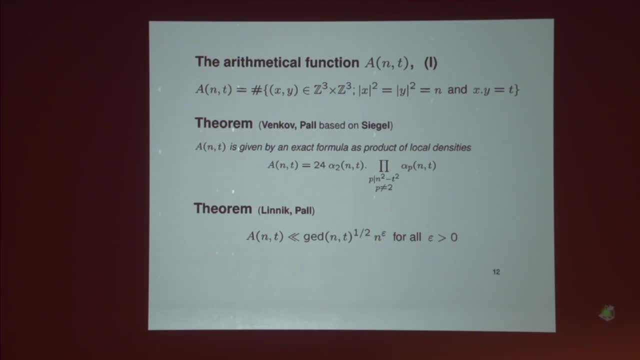 which is Siegel's mass theorem. And Siegel's mass theorem allows you to express the a and t as a product of local densities, And this was done exactly explicitly by Venkoff and Powell, So I will not explain exactly what are. 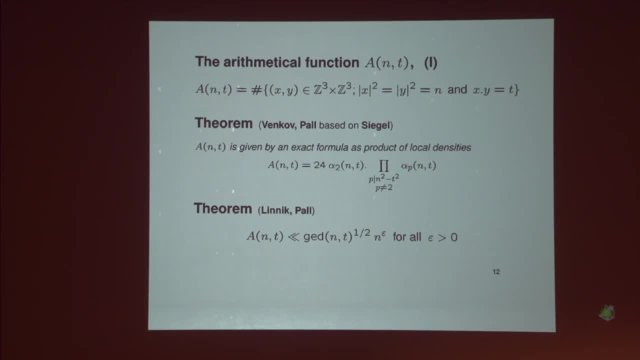 these local densities. but in any case, roughly speaking, it means that you are looking at the same problem but mod p or mod some power of p, So you get these local densities there and then well, that you can try to use. 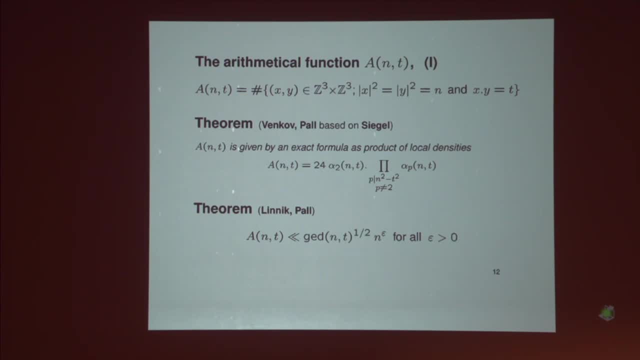 to say something about a and t which is not completely clear. So you get these local densities there. you can try to say something about a and t, which should be relatively clear. So there is a term by Vinnick and Powell. 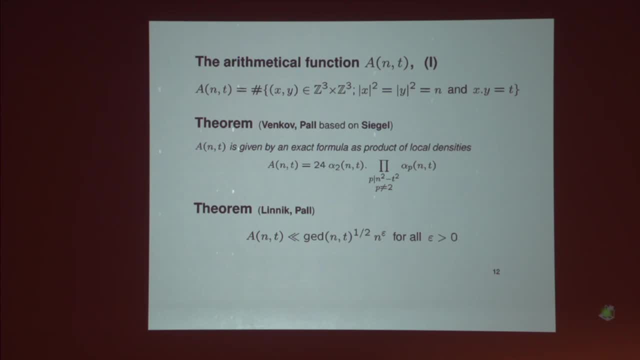 which uses this factorization of local densities to show that at least a and t is bounded by n to the epsilon, or path to a factor which is the greatest common divisor of n and e to the power of r. This is also a crucial estimate in Lenins work. 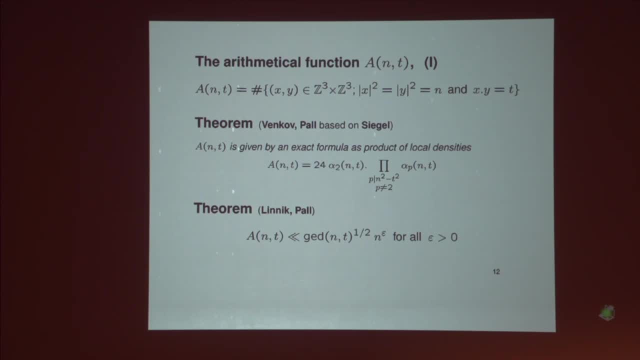 on egg distribution, except that apparently, he had forgotten the first factor, which is the greatest common divisor. Next slide. So, as a corollary, remember that T is not going to be fixed. What we're going to look for are pairs of forms: x, y. 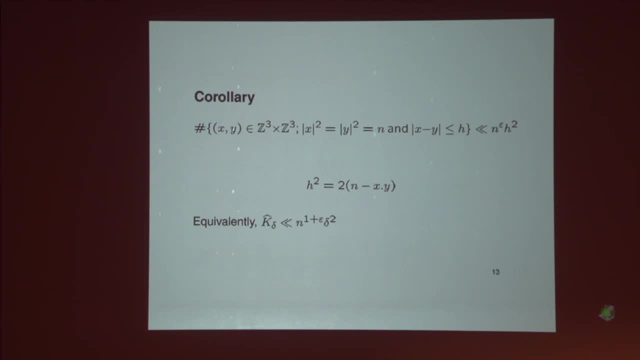 x squared equals y squared plus n, and distance between x and y bound by h, So h squared being 2 times n minus T. What you get is not just the evaluation of a and T, but an average of a and T in a certain range of T. 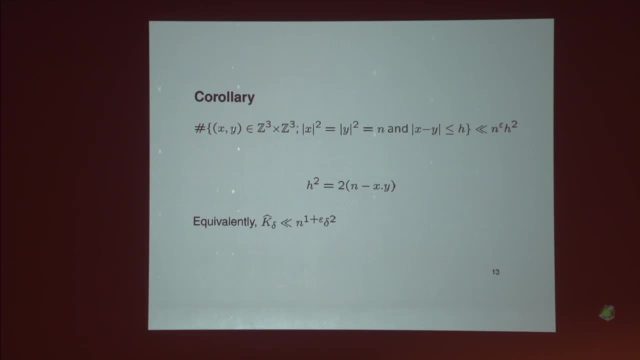 and that allows you to eliminate the effect of the divisor function and show that, indeed, this quantity is bound by h squared into epsilon, which already gives me a preliminary bound on k hat delta which is of the right order, which is n power 1 plus epsilon delta squared. 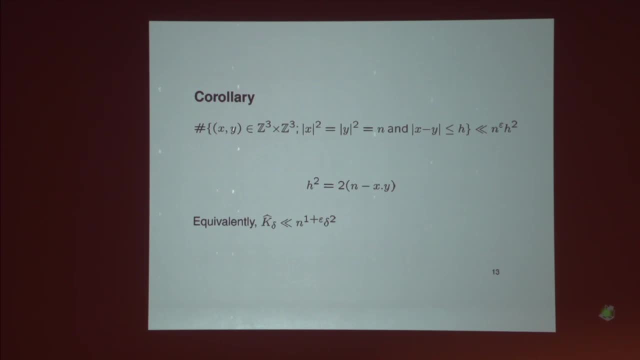 It is not as precise as the one that this projection could be true on the base of the random model, and we'll come back on that. So this is not just the 4 here, 2, but it is already a step in this direction. So at that stage, 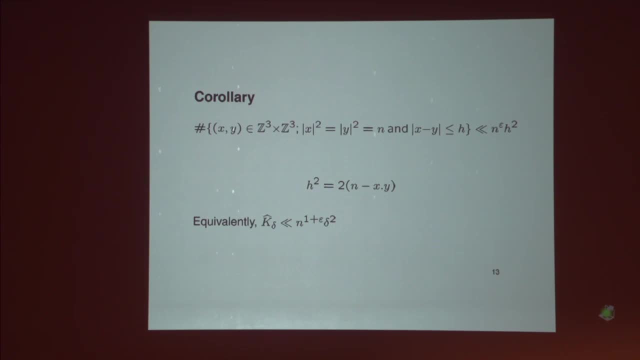 what they have are two things: On one hand, they have the result on the cross distribution, which is given by the Duke Kolubeva-Pomenko, and on the other hand, they have the result that tells me something about large scales, and I can in fact go to some. 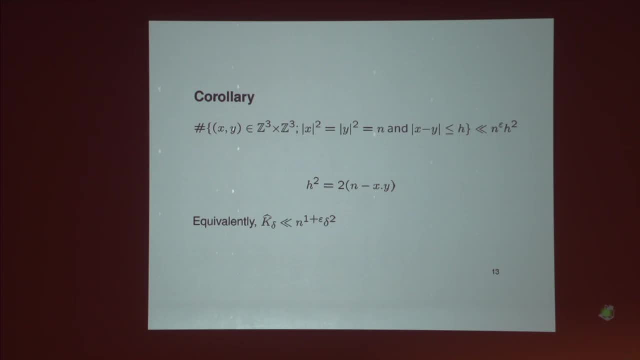 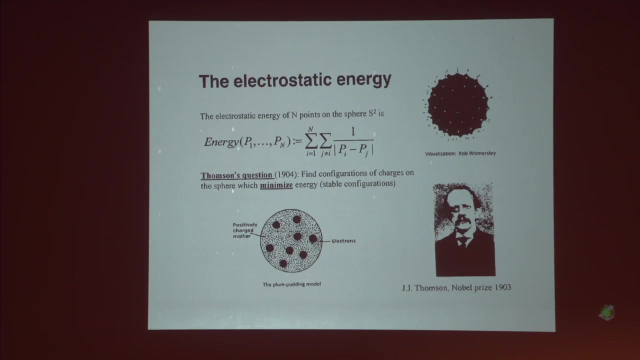 small power of 1 over n. and then I have a result here which is a bound on the liquid function, which is not absolutely exact but is not real and works on all scales. So there is an identification of that to the electrostatic energy. So if we have 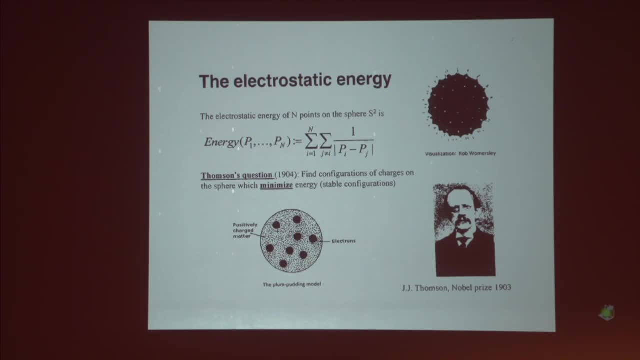 let me recall that if we have a point configuration on the sphere S2, we can define the electrostatic energy as the sum of the reciprocals of the distances between distinct points, PI and PJ. So Thomson's question is the following: find configurations of charges on the sphere? 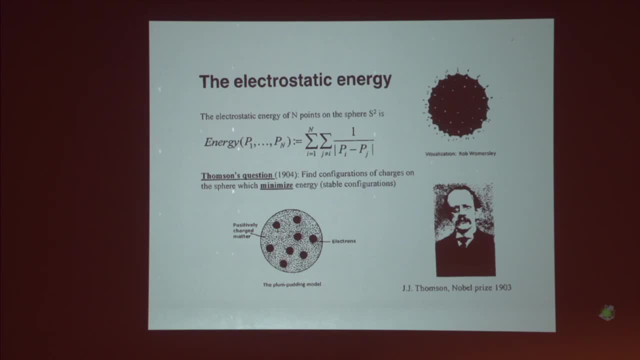 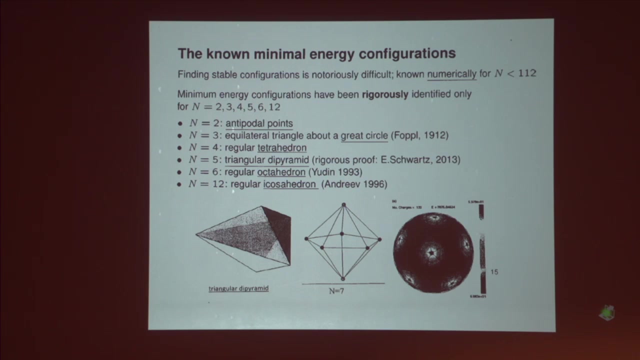 which minimizes energy, and this is something called stable configurations. So stable configurations- understanding is stable configurations- is not real and actually currently it is an open problem. but there are certain things known. Numerically, the stable configurations are understood for n less than 112. they learn from one of my co-authors. 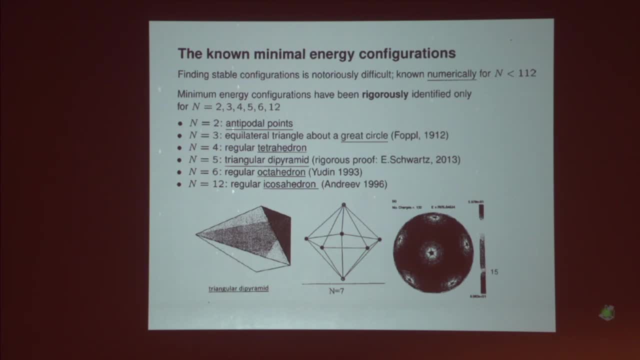 and then rigorously, the stable configurations have been identified. say for n equals 2,, 3,, 4,, 5,, 6,, 12 and so on. The stable configurations, they have certain properties. First, Wagner showed that the energy of a stable configuration 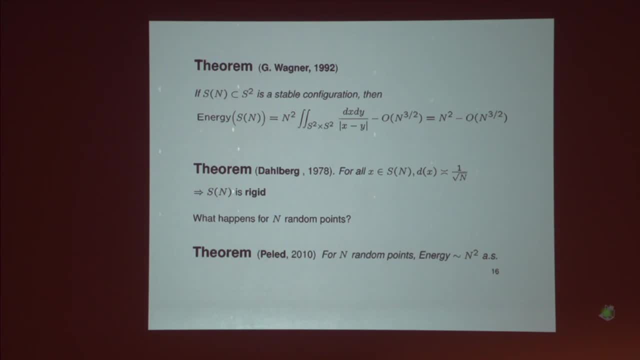 is what you will get from the uniform distribution which would give you an n squared, but smaller by an amount which is of order n to the power 3 halves. Now, stable configurations do not exhibit at all a random behavior. in fact, they are rigid. This is a theorem of Baalberg. 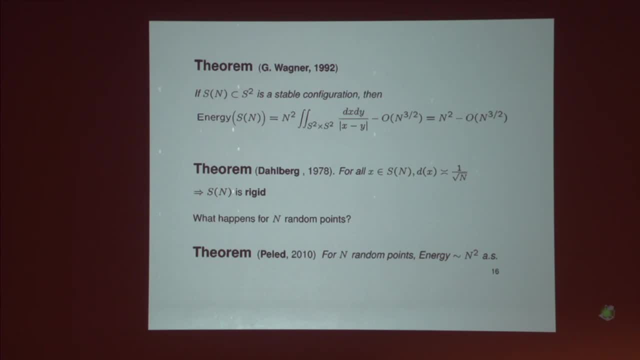 1978, who proved that if we have a stable configuration, then for every point x, the nearest, the distance, the nearest nanodistance, behaves like 1 over square root of n, which is a rigid behavior, not a random behavior. So we can ask what happens in the case. 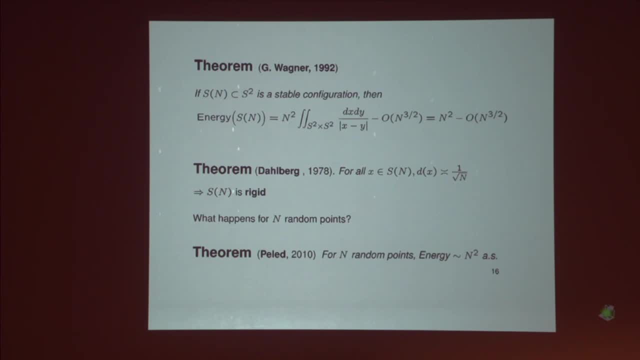 in the model for n random points, where Pellet established that this energy is going to be asymptotically, like the main term here, like n squared. and so now the next question is: what happens with linic points? So with linic points it turns out that the energy n. 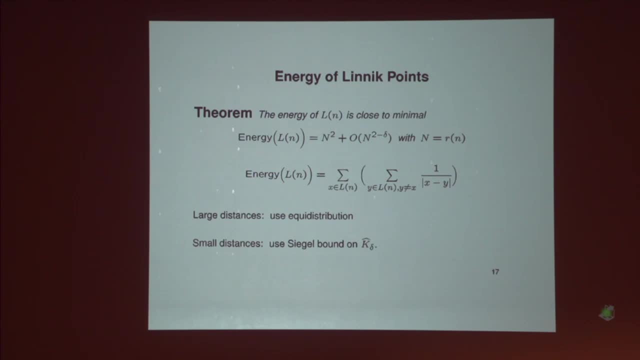 of the linic point configuration is close to minimal, we get in the main term n squared up to a lower power term, and the way this is proven is that. so we have to analyze what this double sum over x and y is now if x and y are separated. 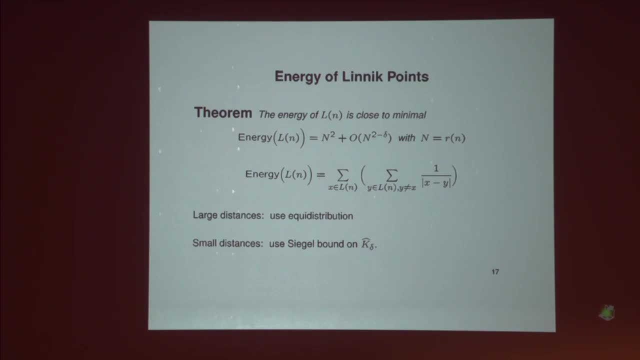 are sufficiently separated by at least n at the power minus delta, we can use the equidistribution results and eliminate the quantitative version, because we have a power gain there. and then what happens when x and y are smaller? well, that could be a problem. that could be a significant contribution. 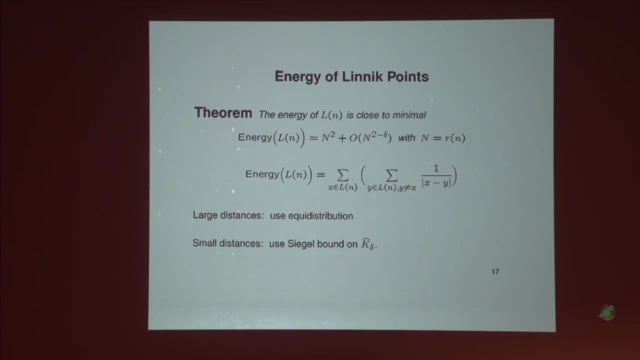 of pairs of points x and y which are closer together. now it turns out that this contribution is minor and to show that it is enough to use our preliminary bound on the repeat function k delta hat, which came from the secret mass formula. now, next, next, we'd like to go. 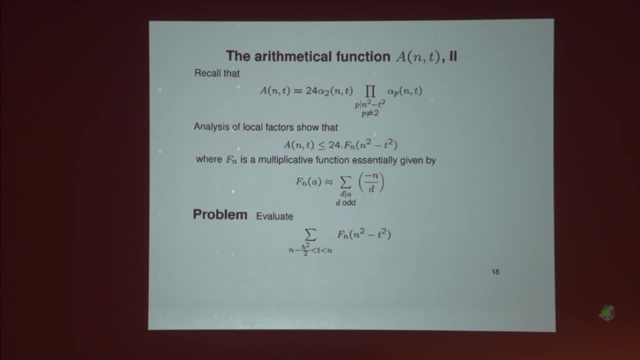 we'd like to come back. try to prove something. try to establish theorem two, which is the precise upper bound for k delta. so we need to understand now what is A and T. so the code A and T is a product of these local densities. these local densities can be analyzed. 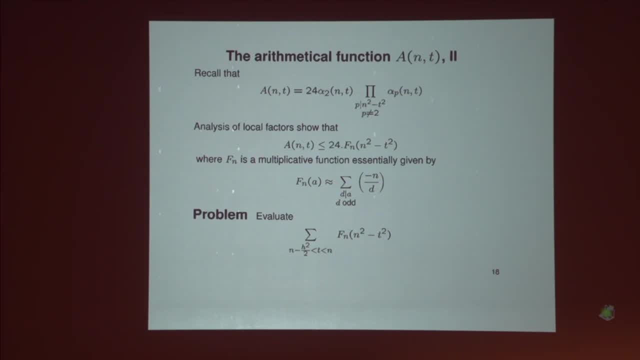 and it turns out that A and T, at least is controlled- is bound by a multiplicative function which is given by the sum of Kronecker symbols minus md. so where so teta A, the function of A, the multiplicative function of A, roughly speaking, the sum of the minus md. 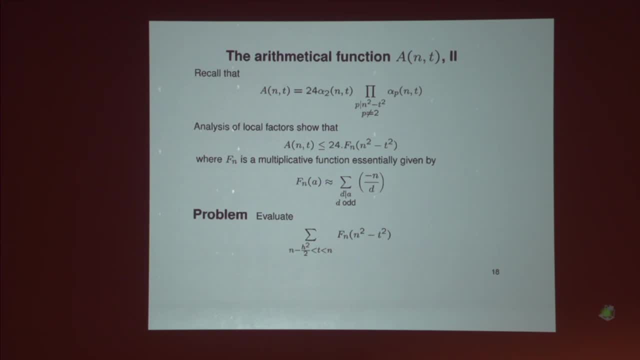 Kronecker symbols of all divisors, of divisors d of A, and that amounts then, when you want to understand the repeat function, what it demands to is that we should evaluate the sum of f, n, n square minus t, square of t in the range n minus a square of 2 n. 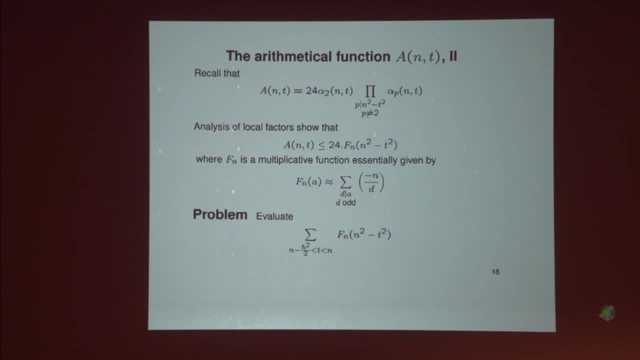 which is an entry level task, but fortunately there is, although we cannot evaluate it. there is another bound possible which comes from a beautiful t level, negative. and what? the theorem of Nair? Nair's theorem is more general. it's the next slide now, so we are considering: 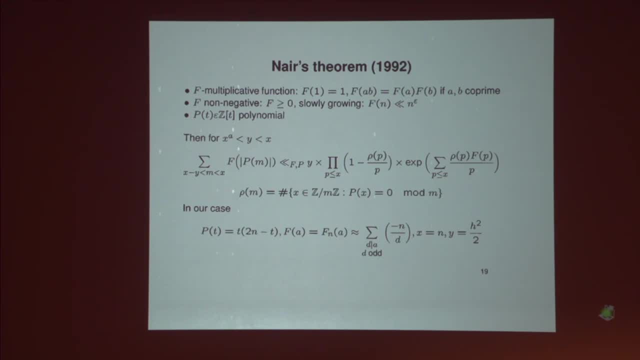 a multiplicative function which is not negative and which doesn't go too fast, then we have a polynomial p of t. so in our case there is a mismatch there. the polynomial p of t is just n plus t and minus t n square minus t square. and we have to. 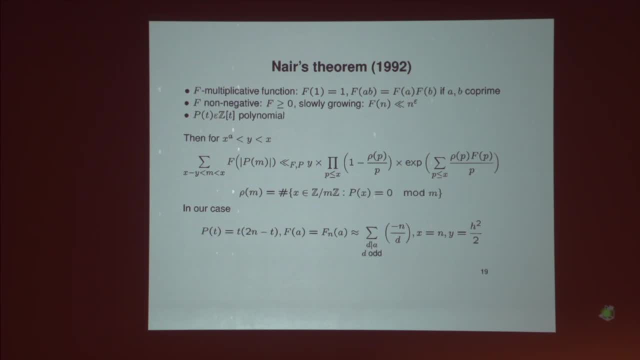 that is exactly the question we have. we have to sum that multiplicative function of the values of this polynomial in a certain range. so the x is equal to n, and then the y is h square over 2. so there is an upper bound which is established partly. 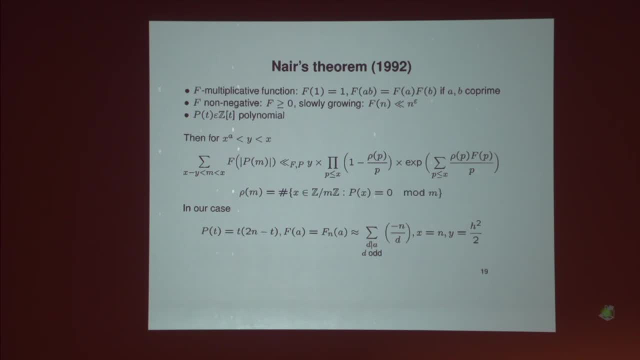 using ideas of ceiling. so the range is y, so we have to get a vector y there. then there is a product of two quantities. the row m is just the cardinality of the x and z mod n, for which p x is equal to 0 mod n. 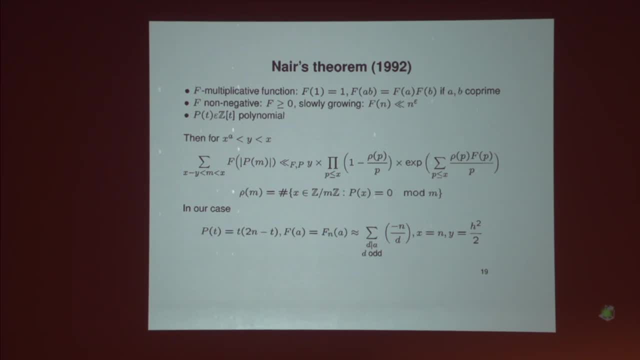 so if you take p prime, because of the product polynomial there is, the row p is going to be basically 2. so we have this first factor, the one minus row p over p, and then the second factor which is the exponent of the sum of row p. 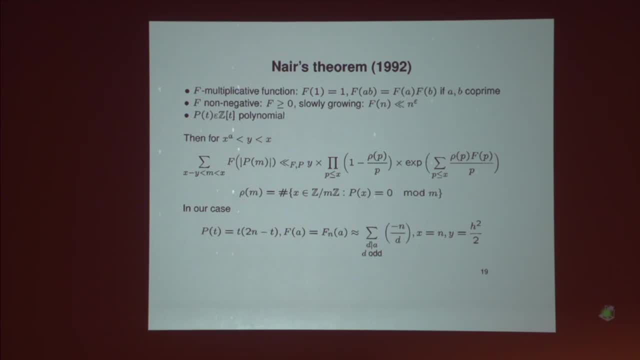 and p over p, for p less than or equal to x. so what you see is that if you take these two vectors together, then basically what this first factor, one minus row p over p, is going to do is subtract from fp. so fp is 1 plus the chronicle symbol. 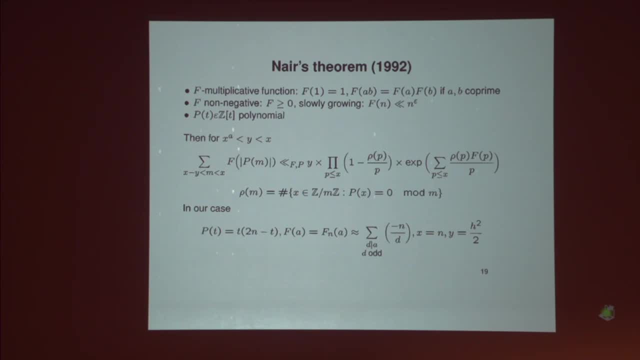 minus np is going to subtract the 1. so basically what you get from this theorem is an upper bound which has the following shape: we are going to obtain that the sum of a and t for t in the range n minus h square over 2 and n. 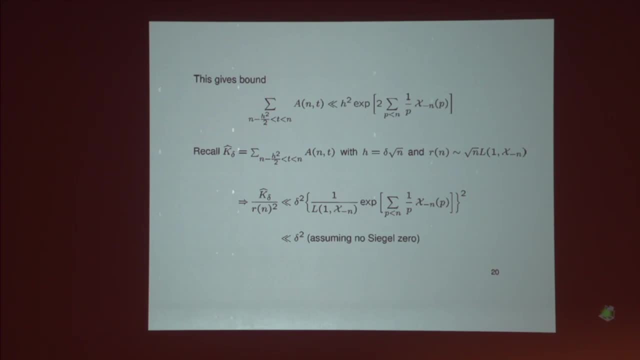 is going to be bounded by h square and then you get the exponention of 2 times the 2 cancels from the row of p sum of p less than n. 1 over p chi minus np. so now the question is how to evaluate the sum in this exponent. 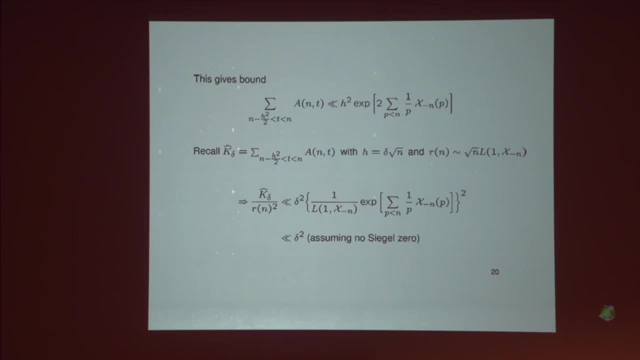 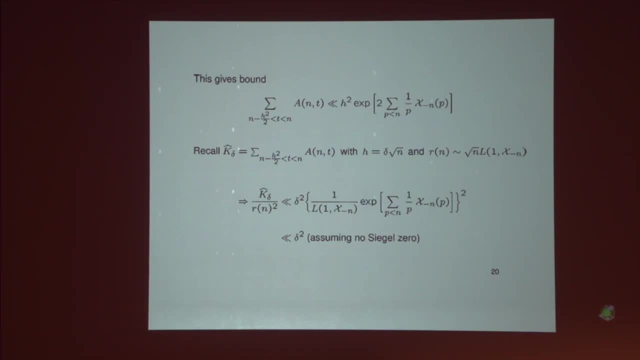 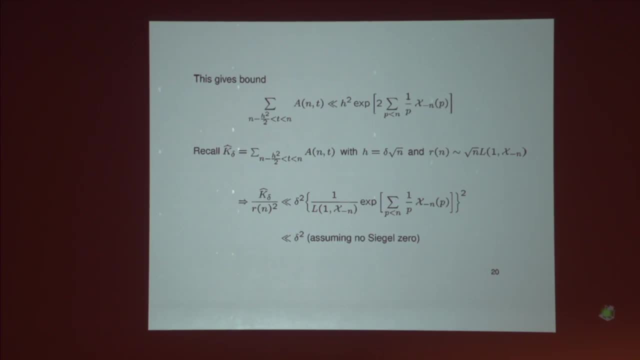 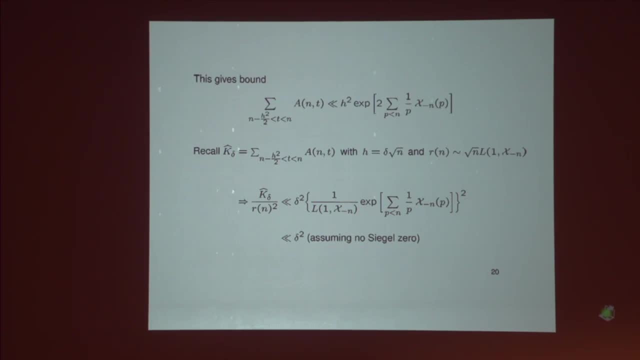 which is the, the right hand side of the first formula, by n times l1 chi minus n. So what this thing is going to give you, keeping in mind that h is delta squared over, n is the expression which is written a second time from the bottom and which involves the ratio between the exponent. 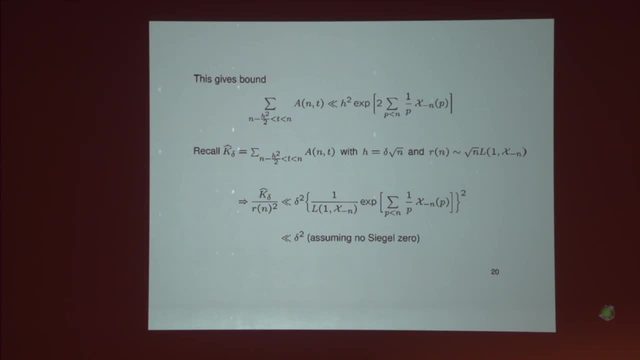 of the sum of p less than n1 over p, chi minus np, over the evaluation of the Dirichlet's function associated to chi minus n at 1.. Now, this Dirichlet's function, evaluated at 1, this is nothing else than the. 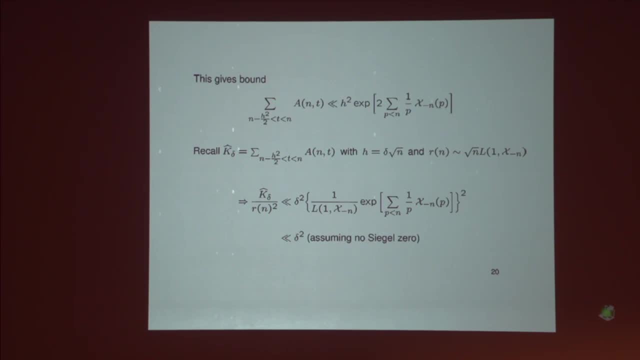 basically it is exponent of the un-truncated sum. So really what we are looking at is the ratio between the exponent of the truncated sum, truncated at n, and the exponent of the un-truncated sum. So in some sense, what needs to be controlled is the sum of 1 over p chi. 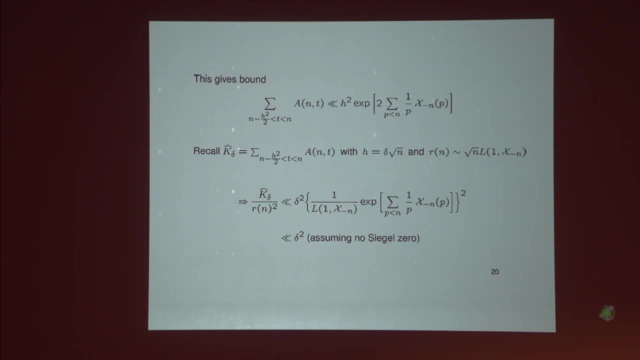 minus np when p is larger than n, And this can be done under relatively un-truncated sum. In the case of the Dirichlet's function, we have zero conditions If we assume that there is no zero. zero means that you get a zero for the Dirichlet's l function, which is very 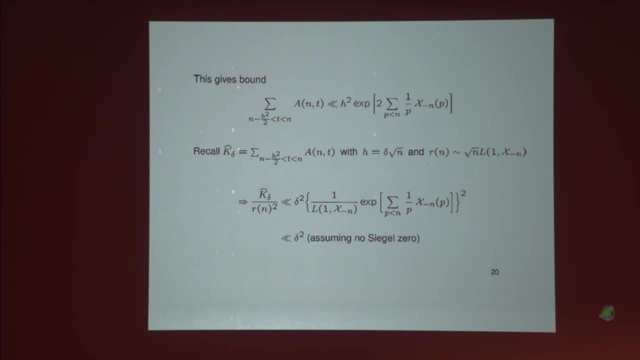 very close to the ring zero, which is very, very close to 1.. And if we don't have that, then we can make this work and, in fact, the expression there between brackets is going to be 0, 1.. Now, the good thing about this zero business is that there is the zero condition. 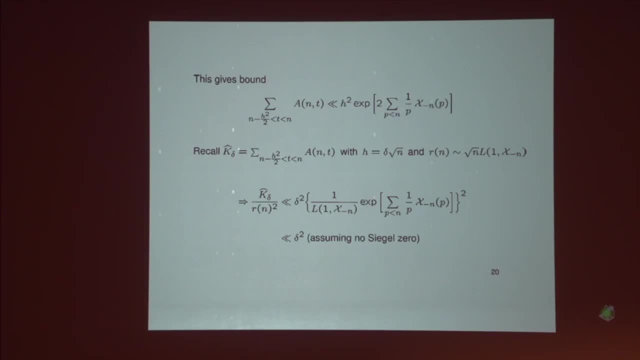 which tells you that if, by any chance, you are lucky enough to have for some n, such as zero, zero, then it won't happen very often. it won't happen. it won't happen for a long time anymore. so there is such an exceptional event that it is quite isolated, which is also 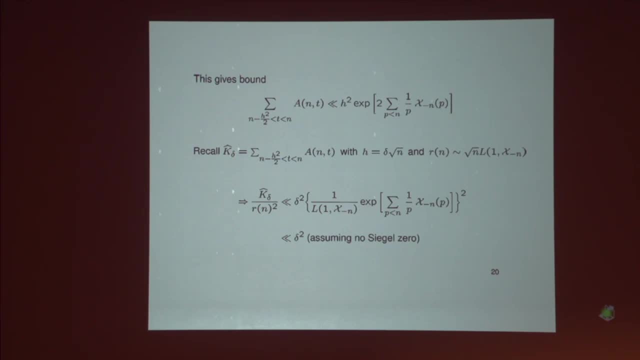 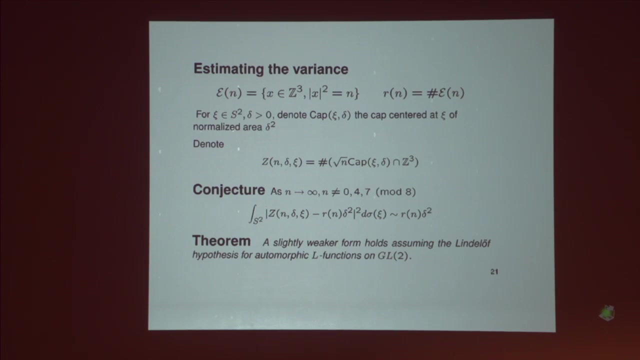 important for the later discussion. so, in summary, subject to the zero, zero assumption, what we're doing is the right upper bound for the reflection. okay, so now i came to the last theorem, and here there is. this is work which is quite recent. we like to prove something about the 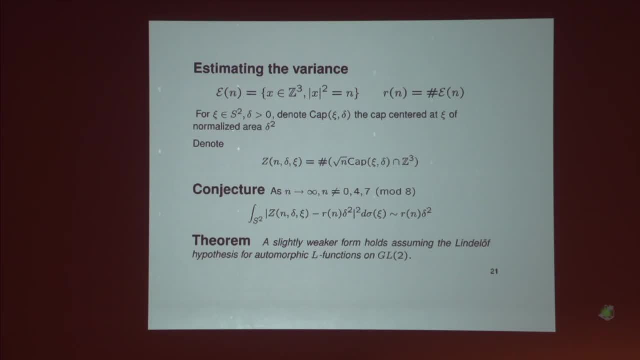 lower bound and what we did. in some sense it's a bit reminiscent of what is done also for the first theorem about the very small spacings, which are the lower bound, and the which i didn't discuss, which is the theorem also about most, and basically to make to obtain. 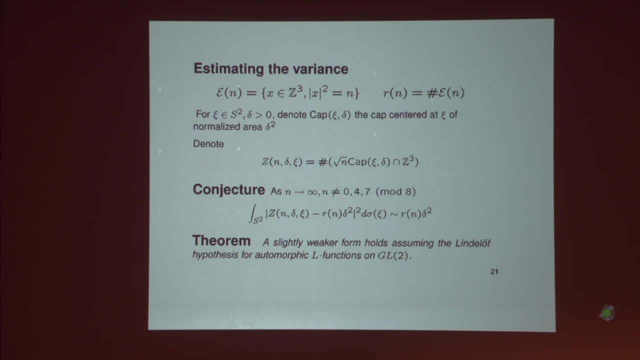 results like that. we are calculating average variances, so let me recall you that we're looking here at, so here we take the, the unknown. i said so. we have the lattice points on z3, x in z3, with x squared plus n and k by m t rn. 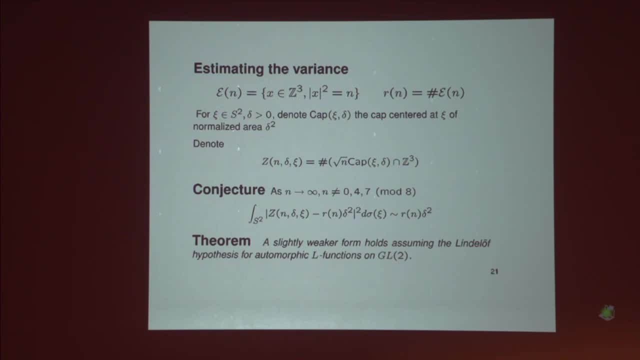 so. so what i will call is cap xi, delta, the cap which is centered at xi, on the unit sphere, and it's not exactly the delta cap, but it is the cap with the normalized area which is delta squared. so then, what we consider are, naturally, that is the thing we have to. 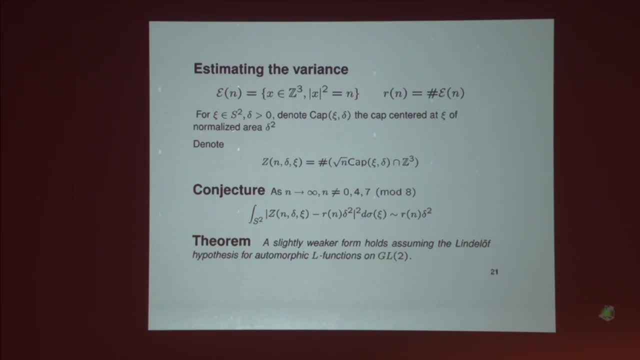 look at the number of points in z3 which are in the cap xi delta and the number of points in z3 which is in case, say we would have good distribution expected to behave like rn delta squared. so the variance means that we are looking at the discrepancy between 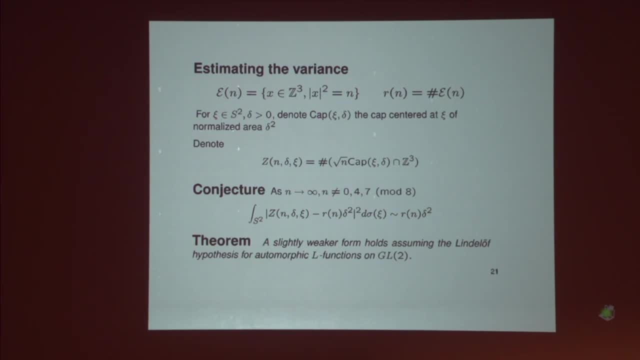 zn delta xi and rn delta squared in average over xi on the unit sphere. so there's a conjecture there that when n goes to infinity 0 different from 0, 4 and 7 mod 8- that should behave the way it should, namely rn delta squared, because that is also what is dictated by the poisson. 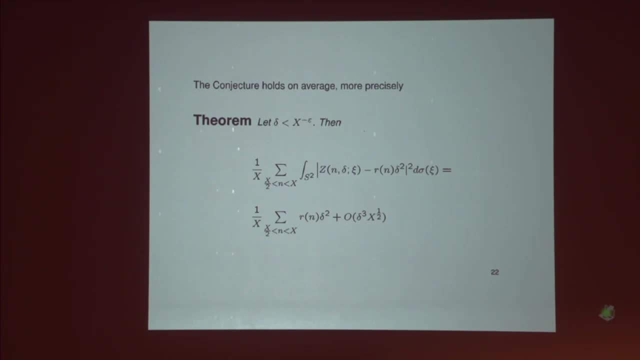 model. now this conjecture is is not proven, but it turns out that a slightly weaker form of this conjecture can be a little bit more effective than the other conjecture. but the result can be proven, assuming the linear hypothesis for automatic f functions on GL2, because 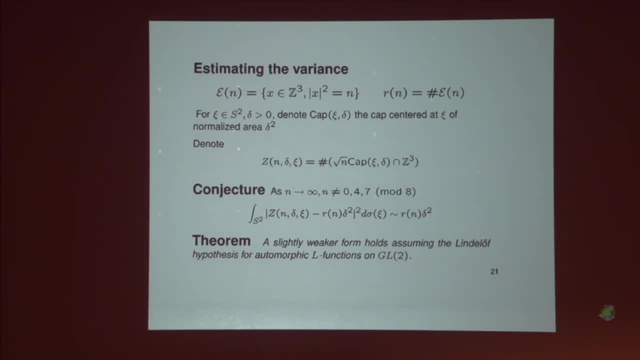 what it turns out is that you can express this variance, you can give an exact formula in terms of harmonic polynomials. and then that expression which involves harmonic polynomials, let's say that we, in fact, can be related to a sum of n and rn, delta squared. so that's. 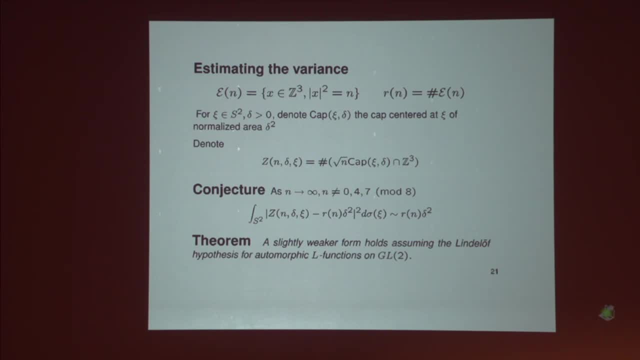 the probability that this calculation is actually feasible. and then you take the same problem of steps in other applications, which is actually a little bit different, except that the Russian hypothesis has the argument that independent function has a function and that electric function has a function, and that is not an equation, is a bilder, a ocean. 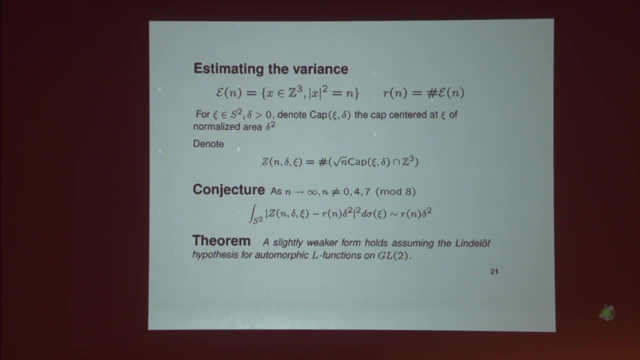 and so on. Then, in a second you see the mind function again and you find that the basis of a certain n function is actually the random function of a certain f function, which is an automatic f function on GL2. and in order to get what you want, you need to make as strong a possible. 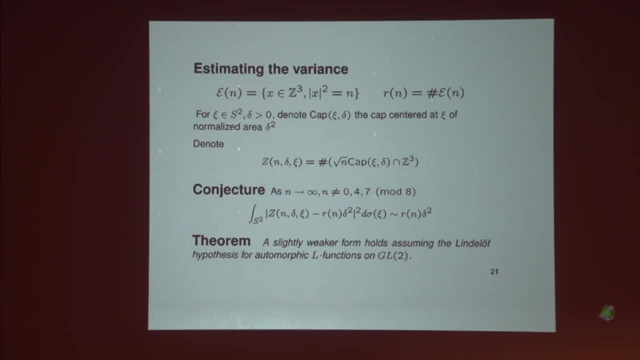 balance on this f function, which is the linear hypothesis. so this is contrary to the conditional result and was mentioning earlier about the z equal to 0. this is a very strong conditional statement and, well, one of the reasons we have is that it's very different from the previous. 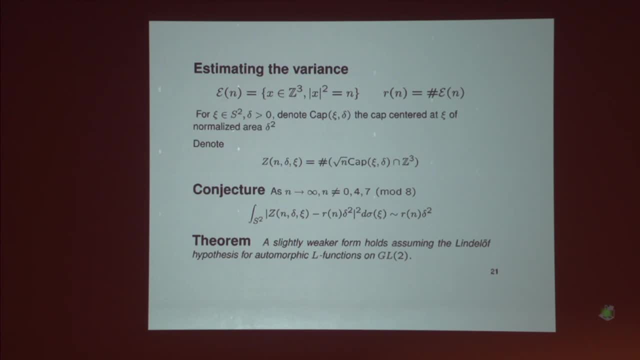 One of the reasons I was going to this work in progress is that fortunately it is not just making an estimate on a single L-function, but we have a family of L-functions there because we are varying the harmonic polynomial. Possibly we could do something which is less conditional in average, as required for that question. 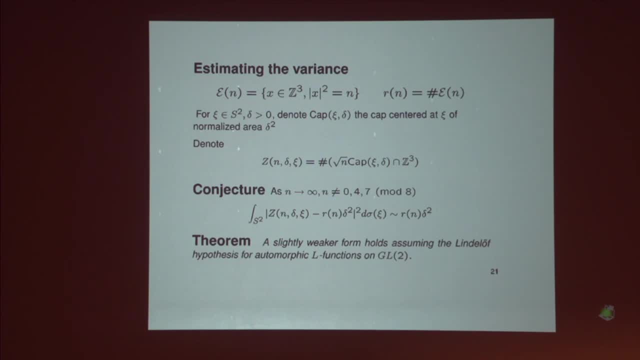 Now what they will do is prove this conjecture in an average form, where we make an addition average over n, and in fact, in a very precise form. So what it turns out is that we have the exact random behavior for the average variance. 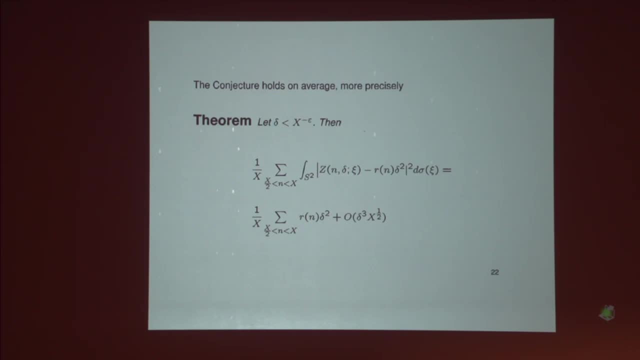 And this is a theorem here, This is one. This is one of the more recent results, So I assume that that is sufficiently small. So we are taking this variance and we are averaging in a range n, say over 4 to x, and we are getting exactly what we want, except for a narrow term which is insignificant. 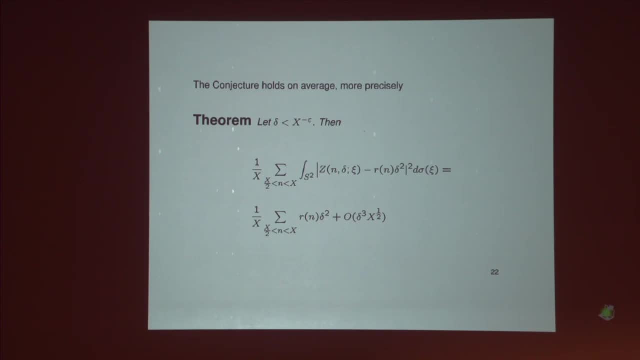 So the proof that result is much more elementary, but still not quite true. So what they want to do is derive the consequences of that statement, in particular The reason why theorem 3 is correct, and it needs the very precise formulation of that theorem. 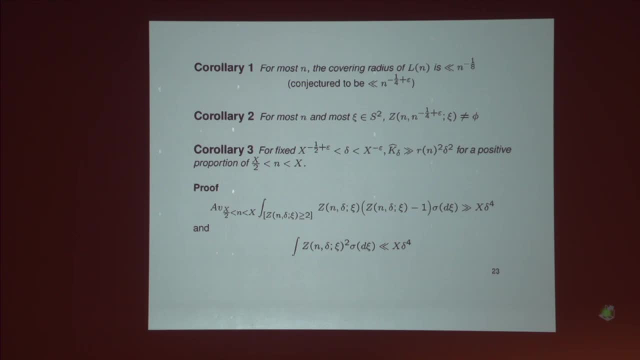 So the first consequence of that result- this is something I did not discuss- what I was discussing, discussing our minimum distances, I was not talking about carrying radii. So the conjecture is… is that the capping radius for leading points is going to be what you expect, namely n to the power of n as a quarter plus epsilon? 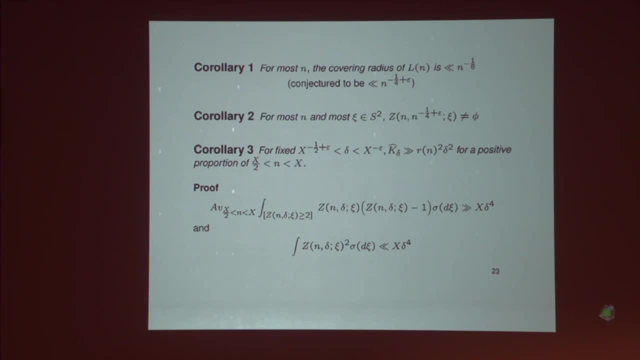 which means that every cap of size n minus a quarter should contain a leading point. So this is something which is extremely hard to prove and it's not even known to be true for most n. What the average variance result tells you is that we get an average, we get a capping radius. 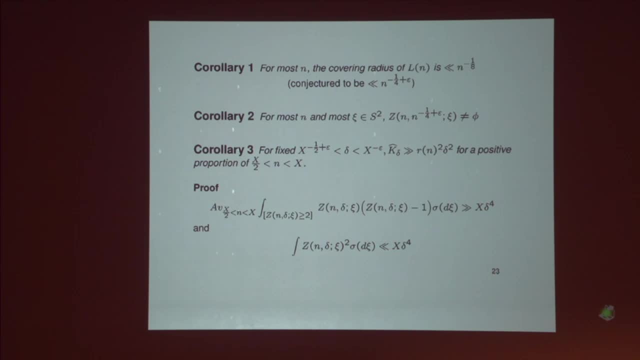 so for most n we get a capping radius which is down to n, to the power of n is 1 over 8, so that is slightly larger. On the other hand, we can be a little bit less demanding and instead of talking about a capping radius, 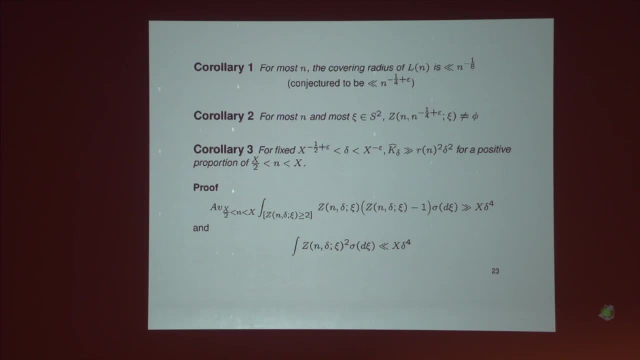 we can do this. We can talk about an almost capping radius, Almost capping radius, meaning that if we say that for most caps of that size, instead of requiring all caps, we can require most caps, most caps of that size are going to contain one leading point. 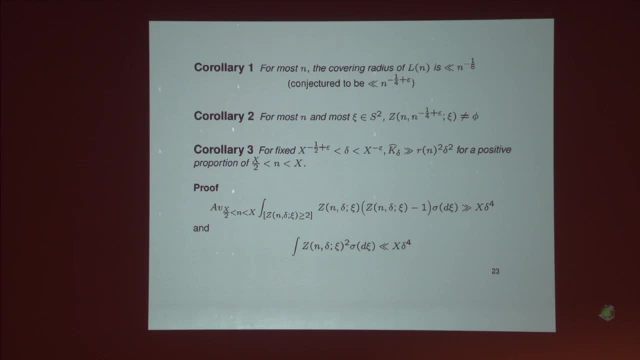 So what the average variance theorem tells you is that, indeed, for most n, we're going to have the. So, for most n, we have an almost, capping, almost capping radius, which means almost capping radius down to the amount that we expect, which is n minus a quarter. 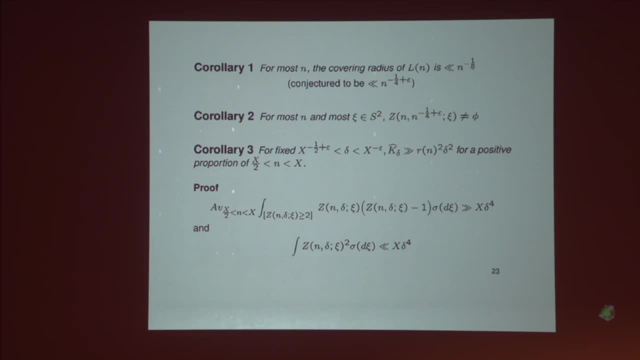 which means that for most c in the sphere, this n minus a quarter of the specimen c is not n. Again, if we would, If we are willing to, If we are willing to assume that in the red hypothesis for automatic GL2, for the GL2 L-fractions, 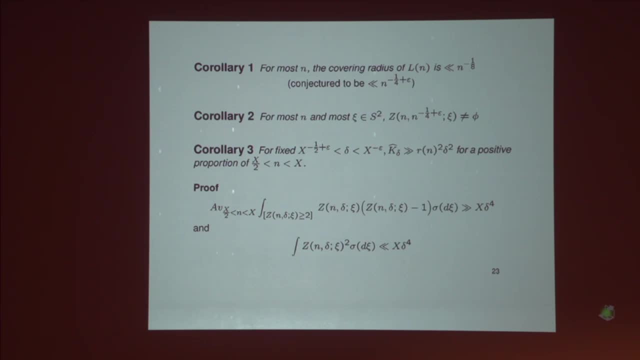 then that same probability 2 would be true not only for most n but also for all n say different from say n different from 0,, 4,, 7, not 8.. So, So, So the same statement would be true without the restriction, without the extra statement, for most n. 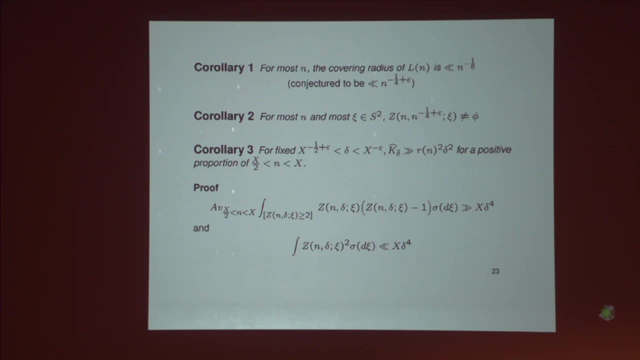 So what would be true is that for all n specified for most c in this 2, the corresponding cap of size n minus a quarter of the specimen would not contain any part. but that is the corresponding condition. That is the corresponding condition. Now to come back to theorem 3.. 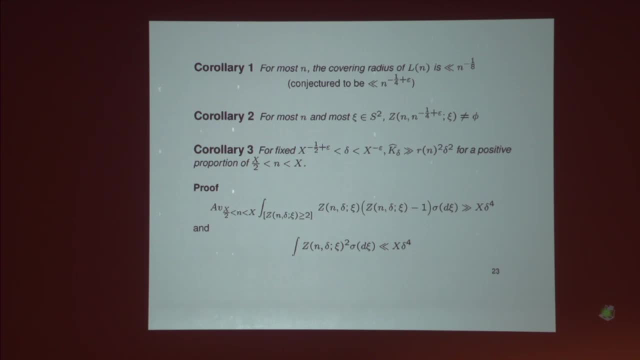 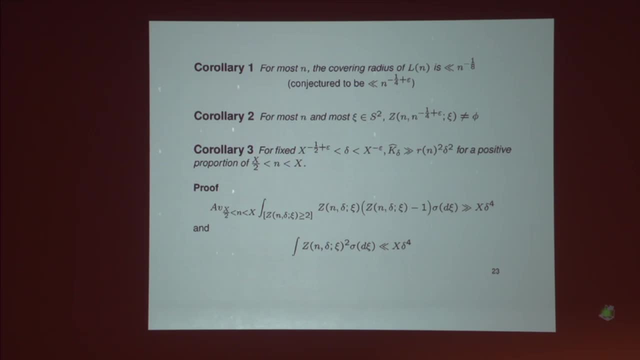 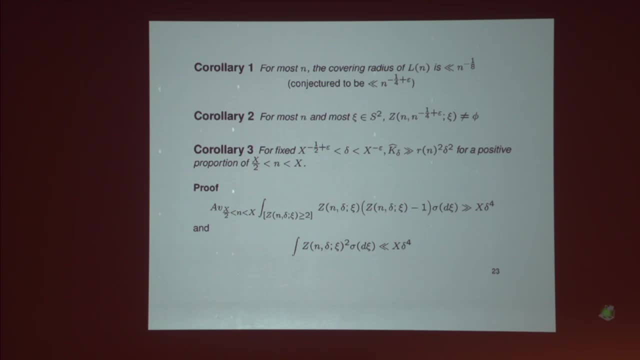 it would just affect one value of n and match. it wouldn't have any effect on the algorithm. So we have that lower bound there, which is the second line of the code, and the upper bound, which is of the same order, and together will tell you. 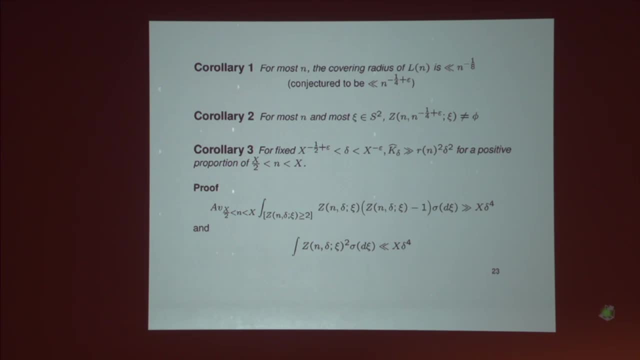 that for a positive proportion of n we are going to have that the integral of z n delta x is square sigma x, z, where z n delta x is at least equal to 2, it's going to be increased on the order of x delta to the 4, and that translates in fact: 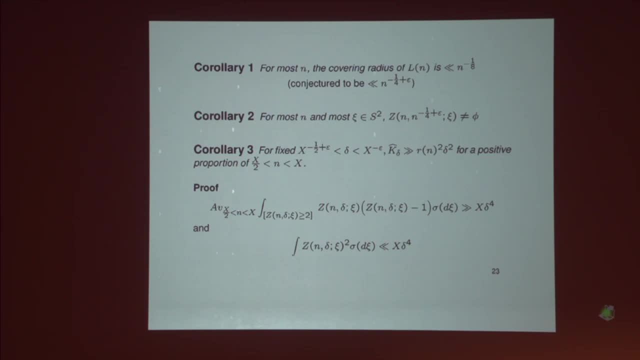 in having the lower bound on the liquid function l? n square, delta square. So what I was trying to convince you here is that there is a certain number of rigorous results that really confirm this random behavior of the leading points, and what is nice about this question is that it is really initiating.